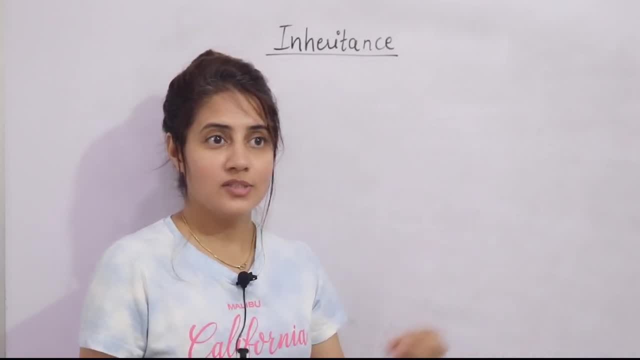 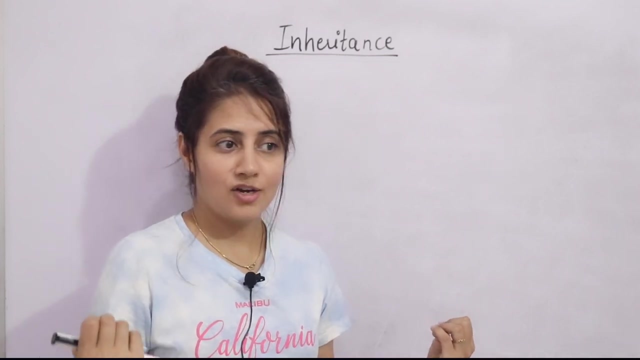 Like this right. So it's our, you can say it's in our genes, Not only the, these properties, not only the appearance, we also inherit the behavior of our parents, Like sometimes, maybe you, you have faced this kind of situation. You just, you know, you behave in a weird way and maybe 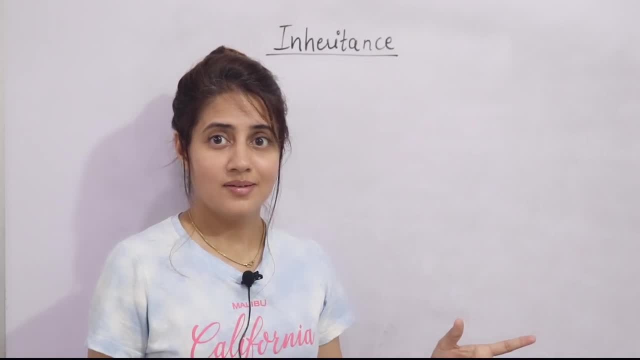 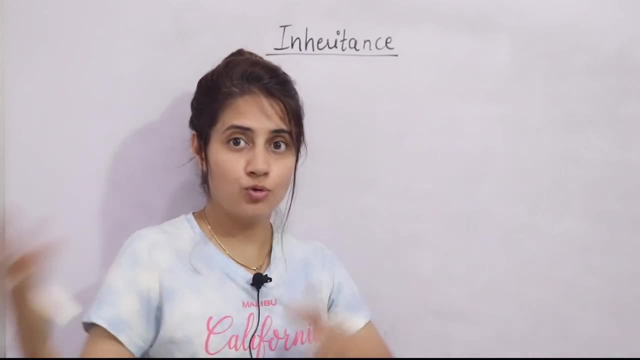 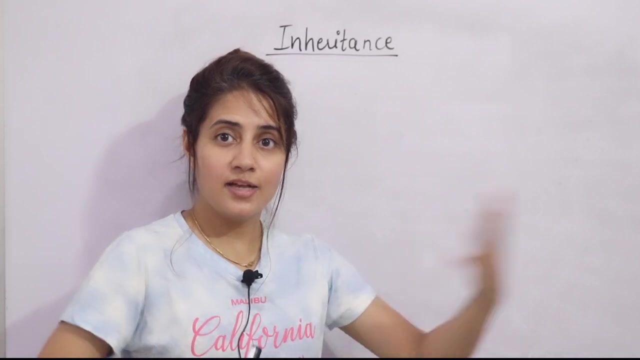 your mother say, like father, like son Means, jaisa bap, jaisa beta. Or maybe your father or your parents are having anger issues. They are short tempered and so you are. You are also are having anger issues. You are also short tempered. You also react same as your parents or your father. 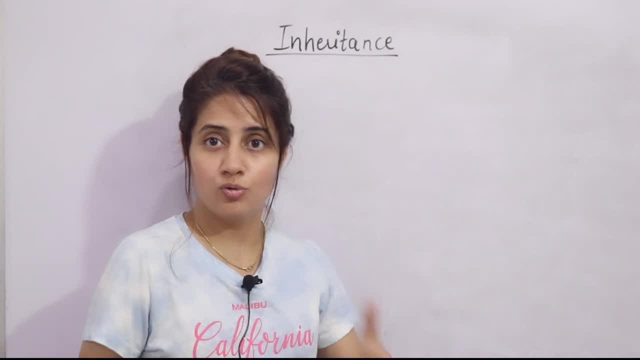 or your mother behave, you know, in a particular situation. You also, you know, react or you also behave in that situation. Exactly same Means we are inheriting the behavior also from our parents or maybe from our grandparents. right, This is, I think you know. 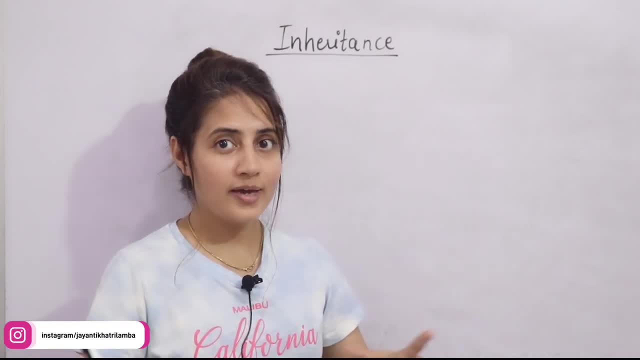 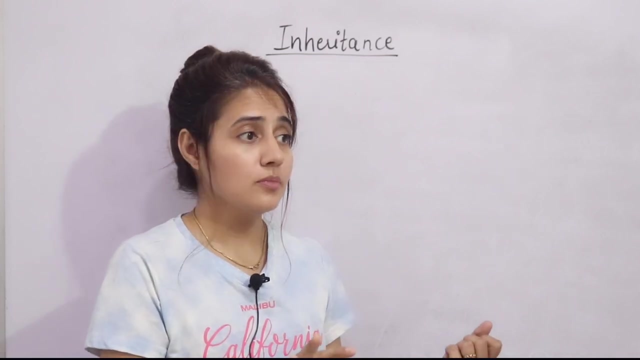 and also you have experienced this thing and obviously you can. right now you can feel this kind of thing. Maybe right now you can feel this kind of thing right. So this is what inheritance in real life. fine, Now this concept we can implement in programming right With the help. 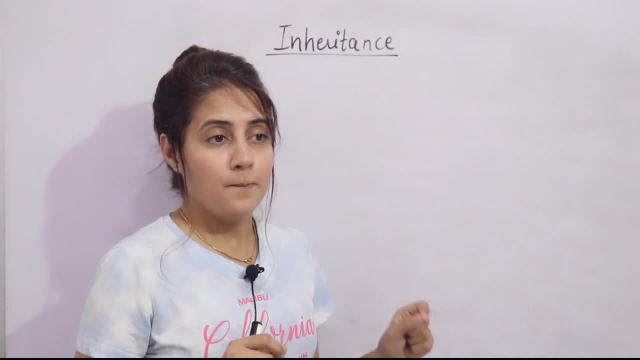 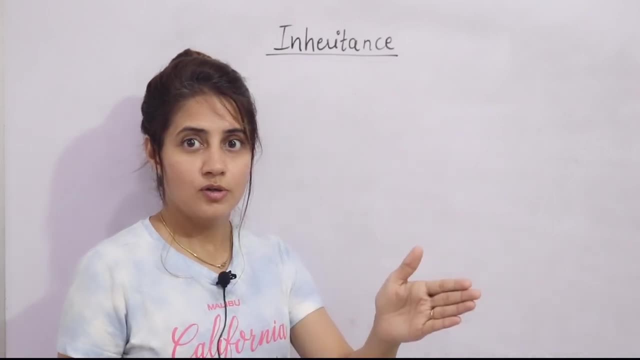 of our system. There we have a concept of inheritance, right Means we can say like: in programming we have classes. Till now we have discussed classes and objects, So classes are just blueprints. Those are having some attributes and methods. And attributes mean: 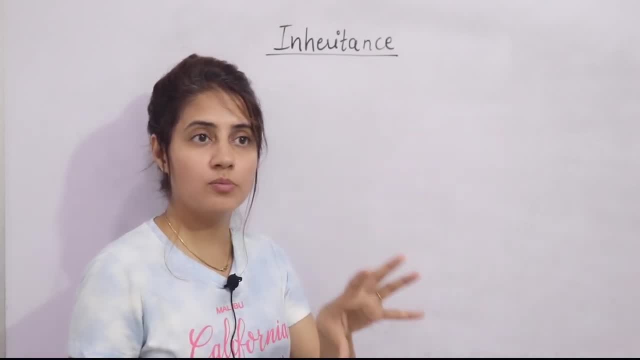 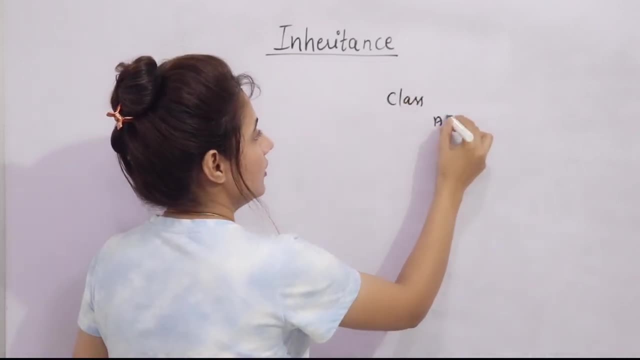 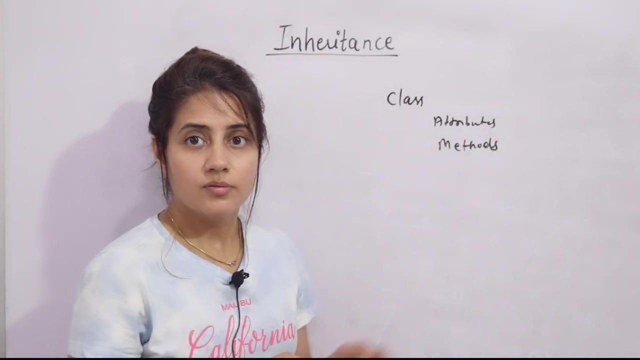 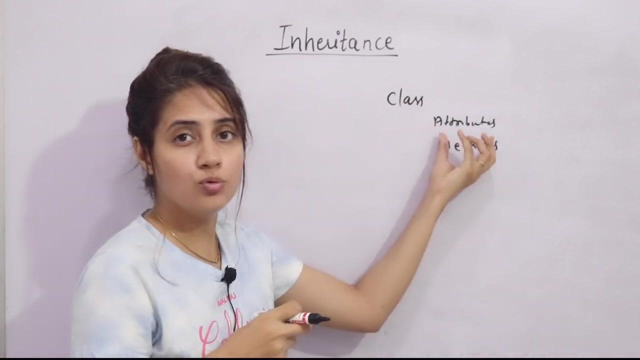 means what? What an object has our attributes? what an object does the methods? Those are methods. So in a class we are having these attributes and methods. Now, when we develop methods right now, inheritance is the ability to inherit the attributes or the. 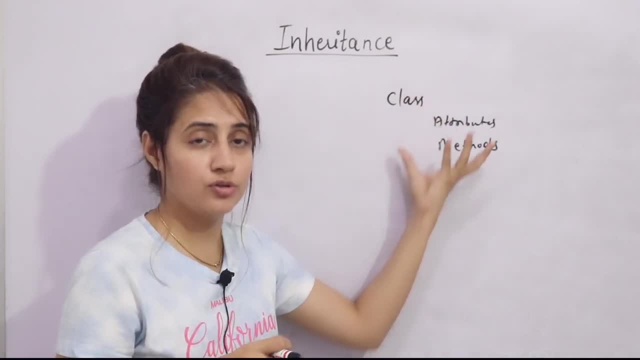 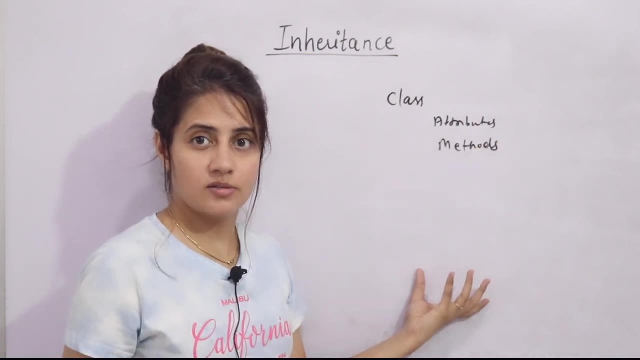 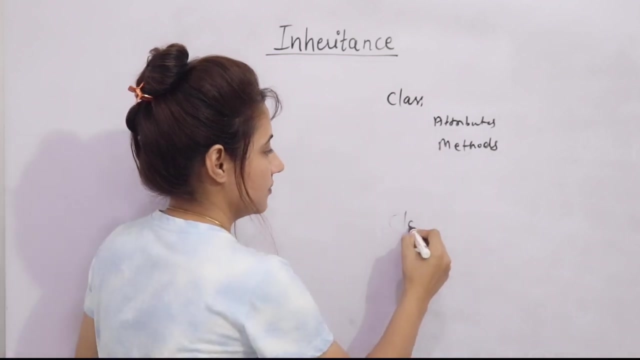 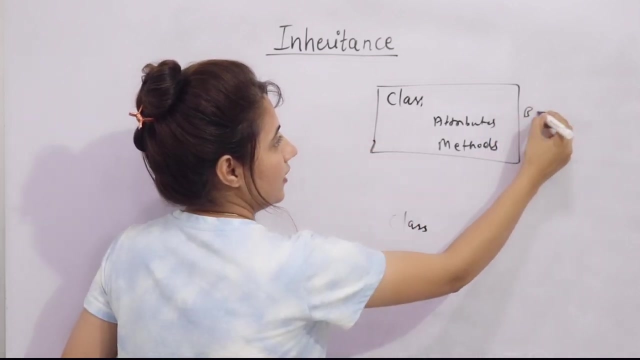 method so you can see the properties of the class or the features of the class already created class to a newly created class. we can inherit all these attributes and methods from this class into another class, so this class is. this is basically from here we are inheriting these attributes and method, so this is. 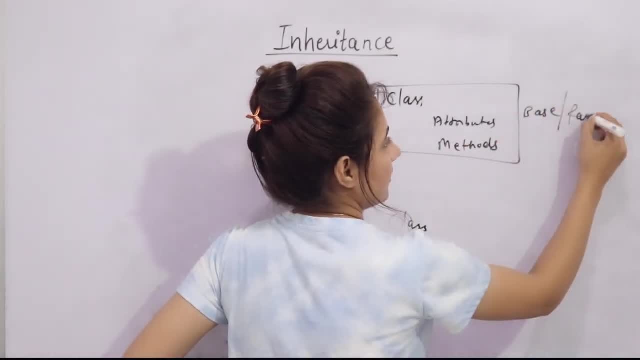 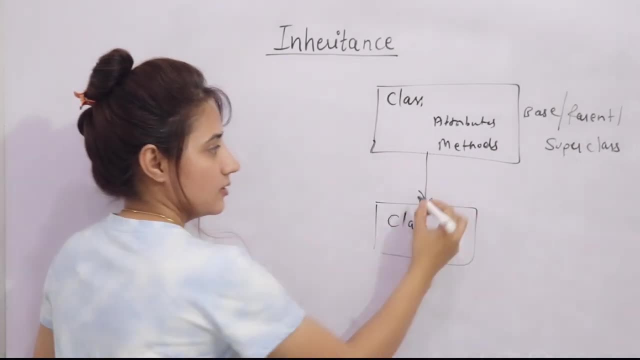 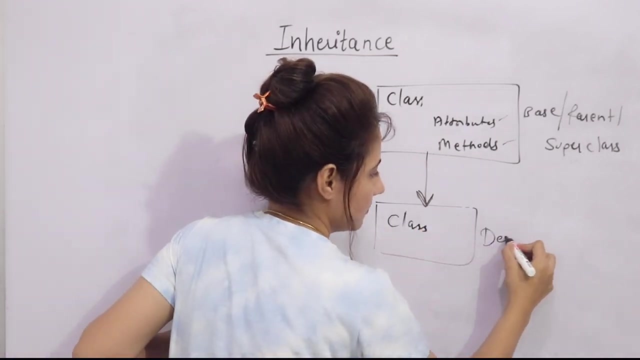 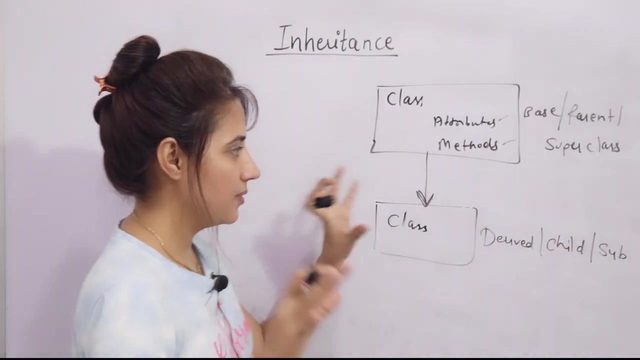 known as base class or parent class, or super class and the second class, which clean hair. it see, we've inherited these properties Illustrated and a metals from this class, this list list known as drive class or child class or subclass, right, so this is simple. you can say inheritance. 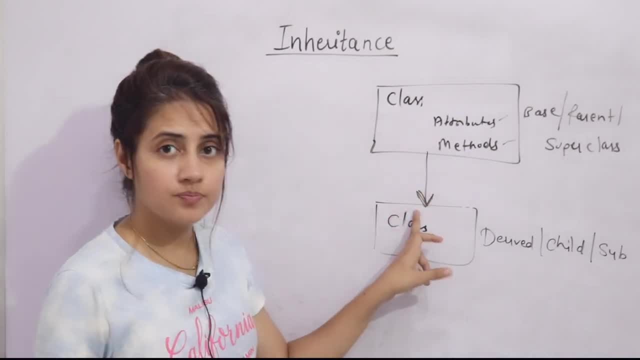 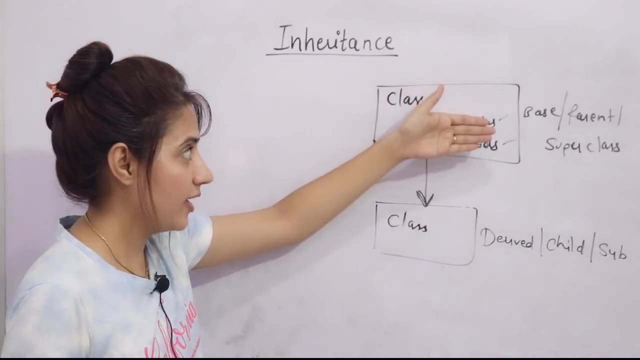 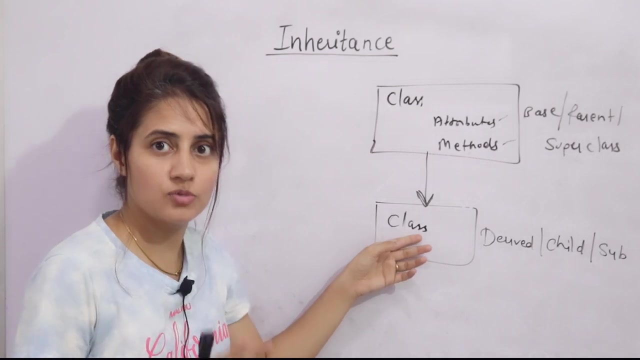 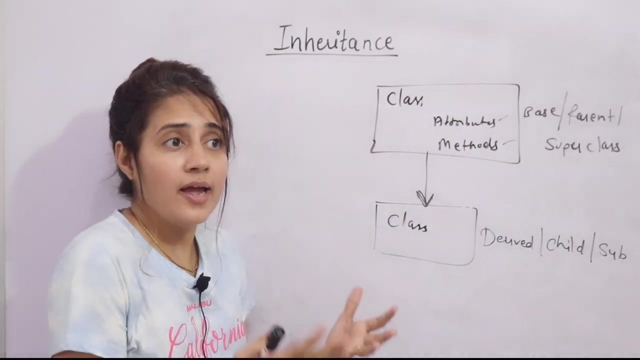 so we can say: inheritance is the ability to inherit the features or the properties or the attributes and methods from an already existing classes or already created classes into newer classes that we make right. rather than creating that class from scratch, we can inherit these features. okay, now this is what inheritance? why? why we are inheriting these attributes and methods. 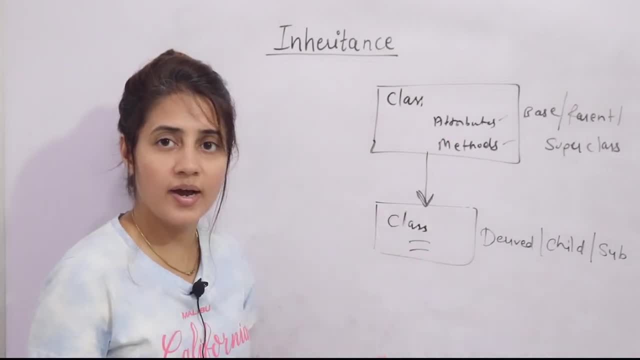 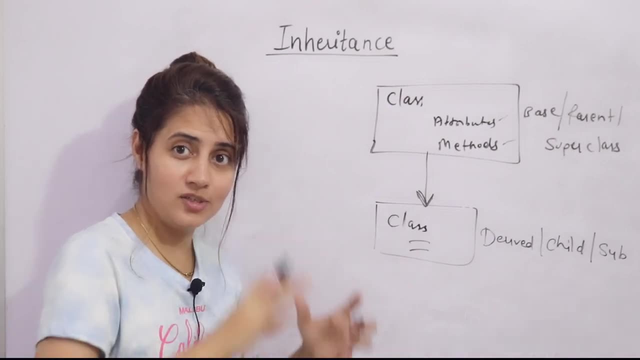 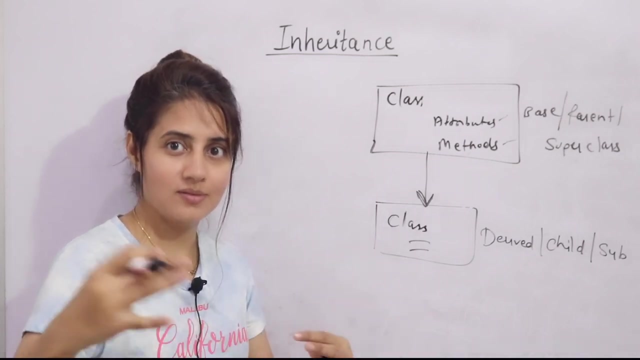 we can also write down our attributes and methods in this class. so why inheritance? the answer of this question is important. so if you got the answer of this question- why inheritance- and you understand this thing, then means you are done almost. you got everything about inheritance. yeah, we are studying many things like types of inheritance and 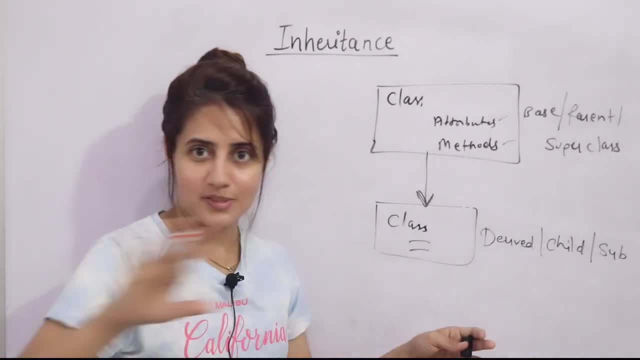 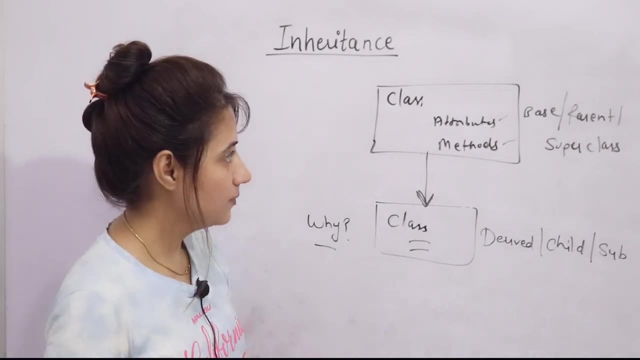 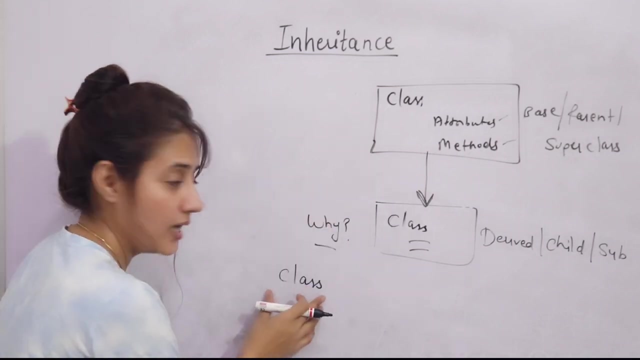 many other things, but the answer of this question is important one before proceeding further. why? why inheritance, so this thing? now i'll see you with the help of program, right, okay, let me just first tell you the syntax before you just write down a name, this keyword class. 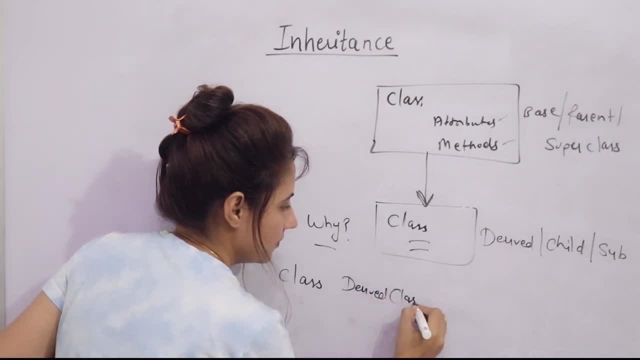 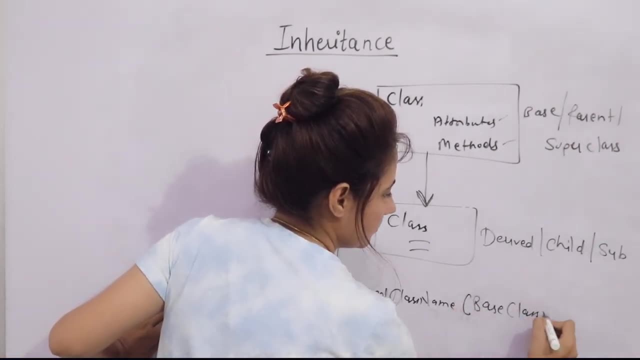 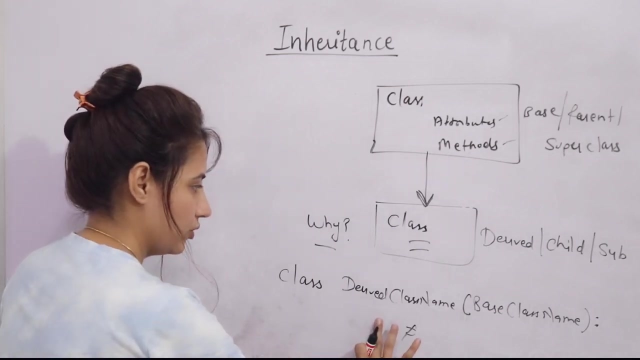 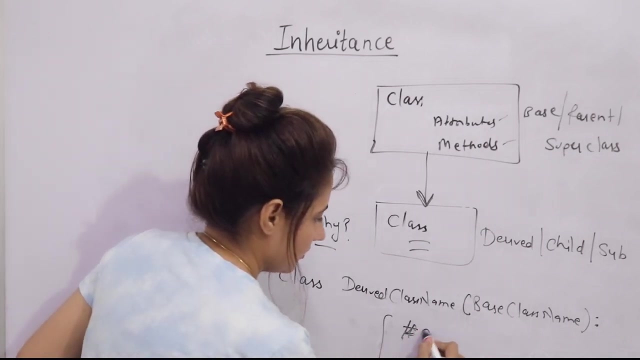 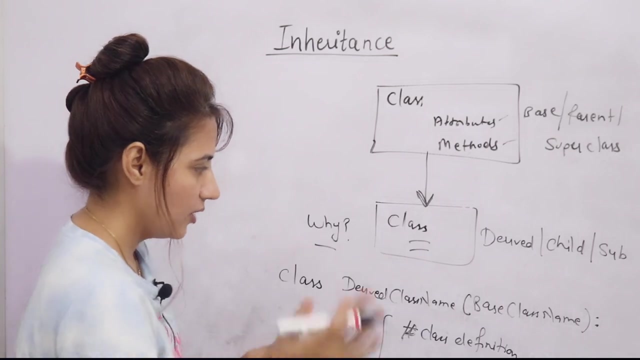 then this drive class name, right, and in break it we write down base class name and in the colon and here the class definition: whatever you want to define in this class, that definition you can write right. so now here you're gonna like class definition or statements. so this is simple syntax of inheritance. now let's see practically okay, so let's create a new file. 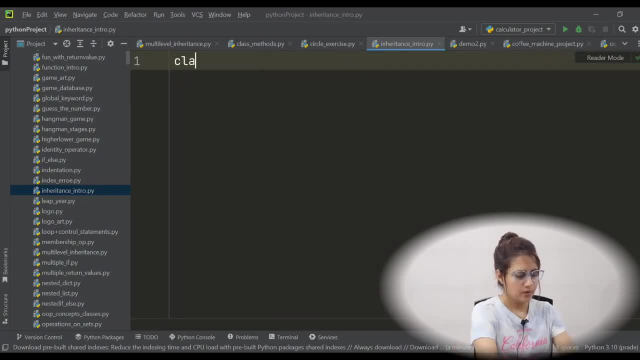 here intro, dot, py, right, I'm simply defining a class and the class name I'm taking like human. okay, now I'm defining some functions like eat and in eat, simply I'm printing like I can eat. and one more function, suppose I'm defining like work, right, and simply I am going to print here I can work. so these two methods. 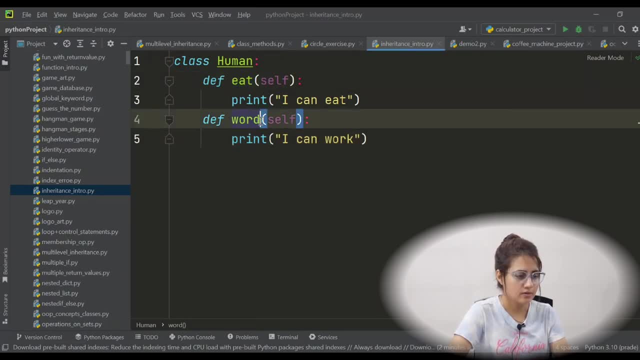 sorry, not function. these are two methods: eat and not word its work. I can work right now. let's define. see, I'm having only right now methods, no attributes. that was we'll see later about attributes. now I am having a class and I'm- and Suppose I am having a class- male. 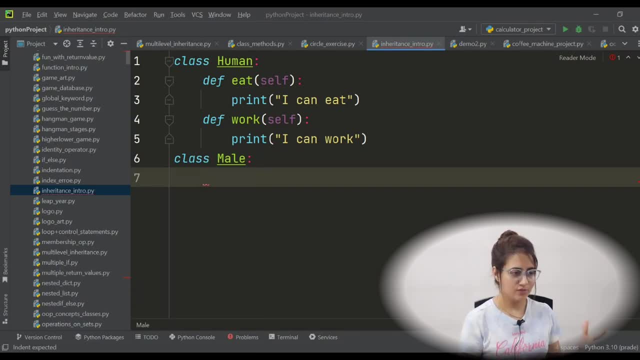 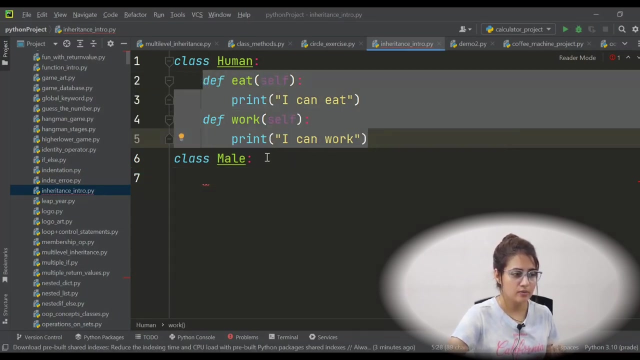 Right Now. obviously all male and obviously females are human being, So male can also eat. We know male can also work Right Now. one way is either in male also you can define these two functions for male and like this, Control C and def- eat. 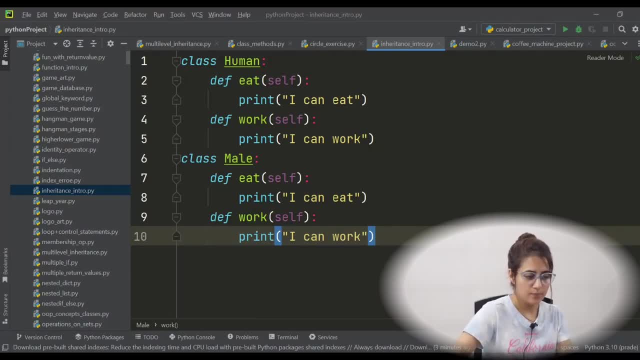 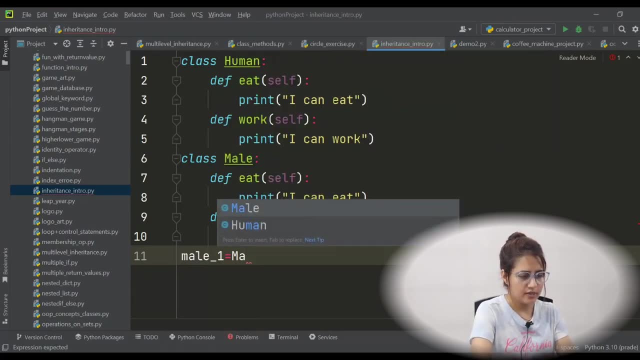 Def work. I can work, I can eat Right And simply if I like, if I create an object of male, male underscore one, any name you can take, and I'm creating an object of this male class Right And with the help of this now male object: male dot C- eat and work. 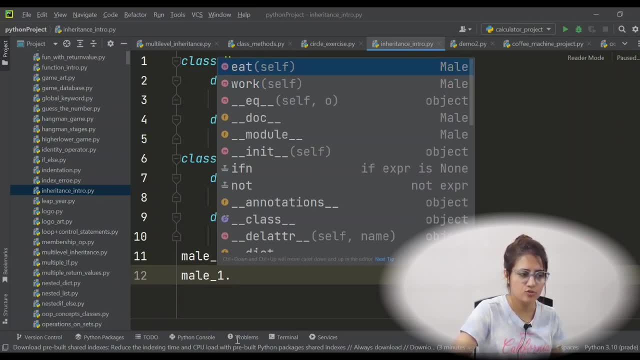 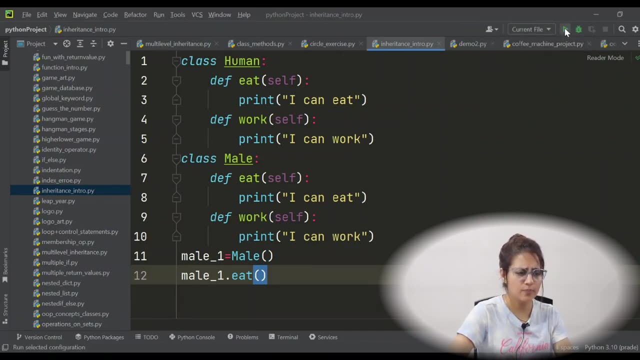 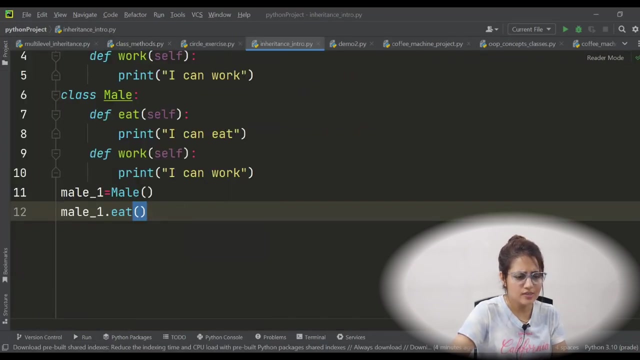 These two methods are from this male and male class, as you can see, Right, So you can access these methods, like, if I access eat and if you run this, then obviously It will print. I can eat C, Right, But the thing is, this is what? just a waste of time. 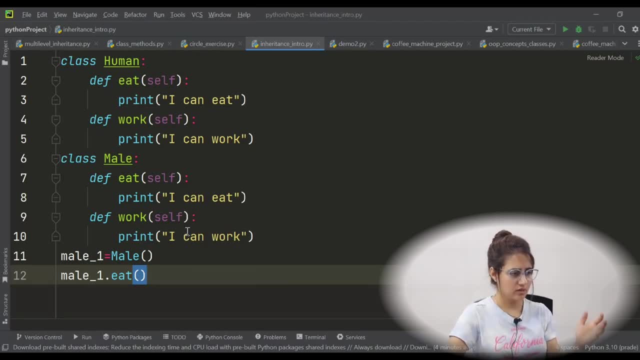 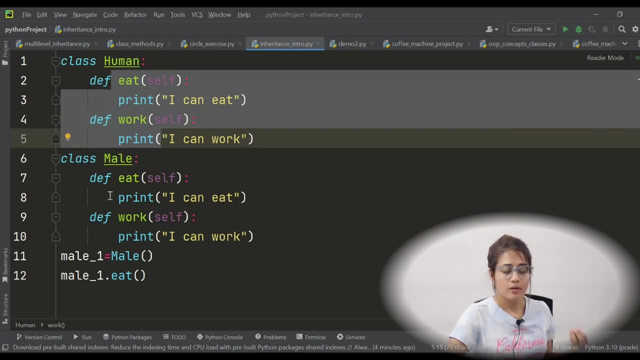 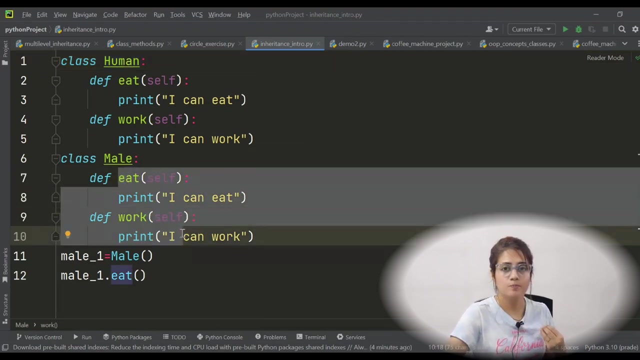 Right And just to increase the number of lines in our code unnecessarily, because we are just repeating these lines, These two things: If you are a human, obviously male are human, so they can eat and they can work. So rather than writing again, I can just use: 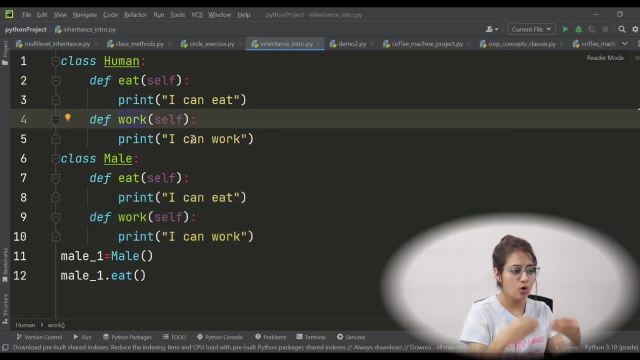 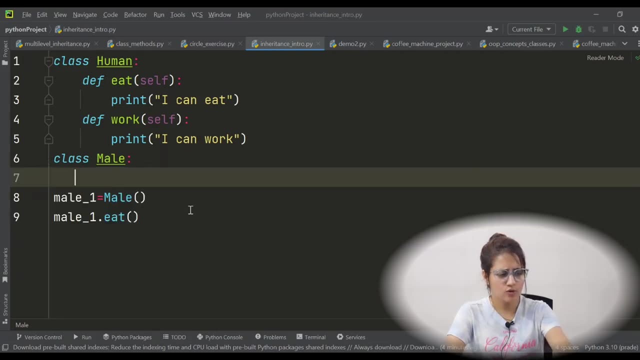 These Methods, These are. these are already defined, These are already in this already created class. So, rather than creating this class from scratch, What I can do, I can just inherit these methods. So this is what inheritance, and this will definitely save a lot of time, because here we are. 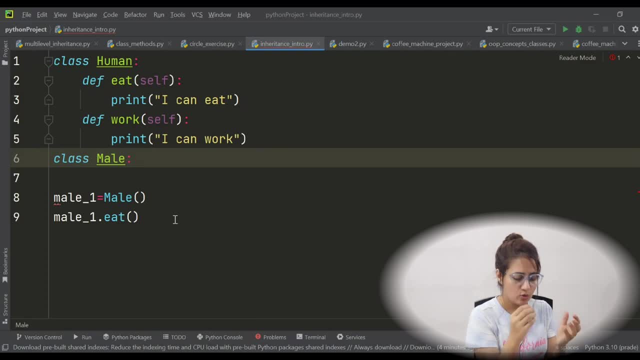 I'm only two classes and only two methods, small example, But on industry level there are multiple classes and very large project on very large project We are working Right. So obviously this is going to save a lot of time and less number of lines in our code. 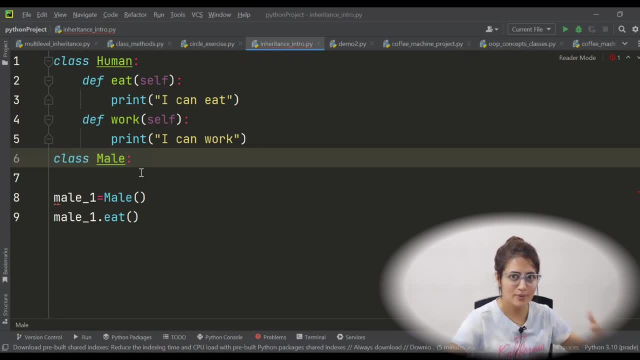 So that is why, if less number of lines, then readability of our code will automatically increase- maintainability as well as readability. Right, So these are. I guess you are getting now the benefits of using this concept. So this is same the answer of why we need inheritance. 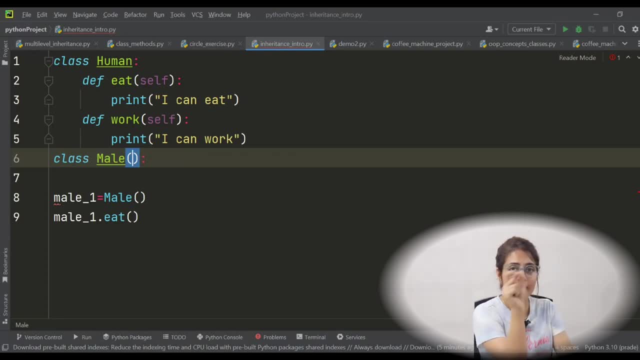 So now, so the syntax. I told you drive class name and in bracket you just have to pass simply the base class. From this class I'm going to inherit these two features, So these two methods. So just write down the name of that class. 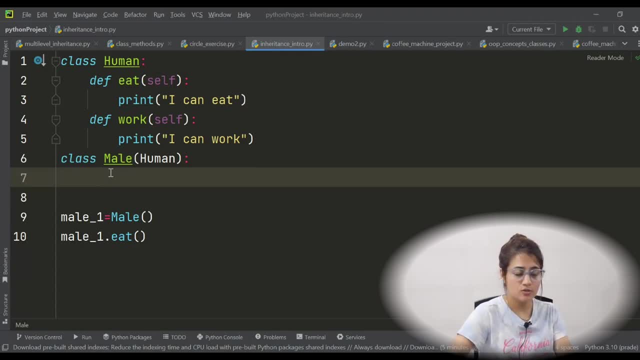 That's it Now. if you don't want to define anything in main class, obviously mail class. if we cannot leave this like this, So just have to pass. Just a pass statement means we we don't know what to write down in this mail class right now. 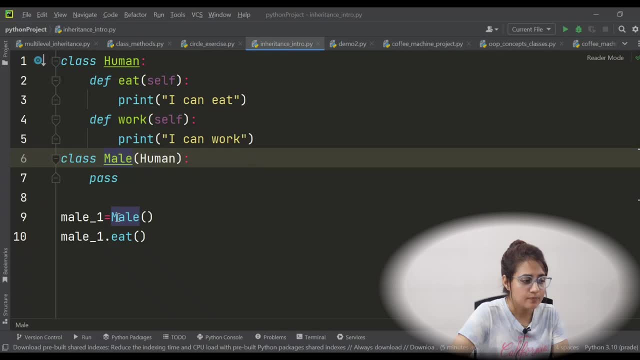 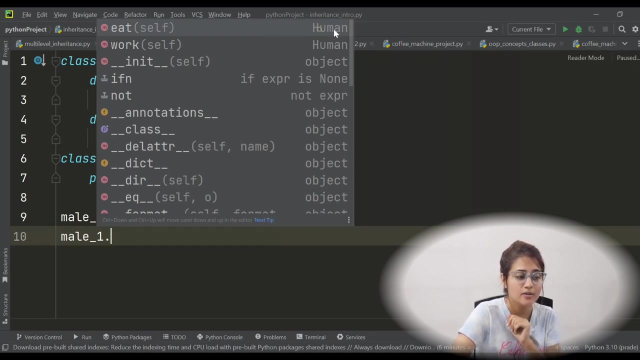 But later on we will define this class also right now in mail. Now see, with the help of this mail object: Mail one Can you access. eat and walk, See Here. also see the difference now, Method: eat and walk you can access, but here see the name of the class, is human. 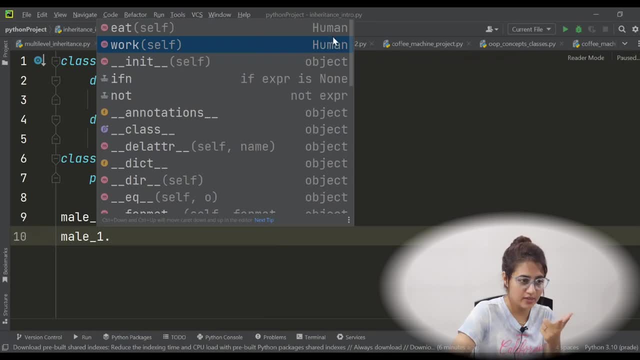 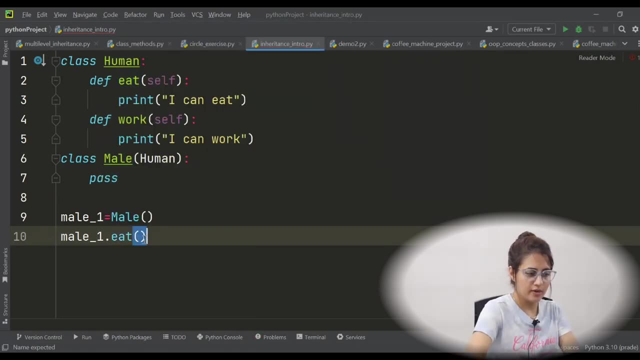 And at previous case the name of the- here the class- was mail and mail. So from human class we are accessing eat and self. So this is inheritance. So now also I can print, I can access eat and, yeah, I can eat. So the main purpose of inheritance is to increase the reusability of the code. 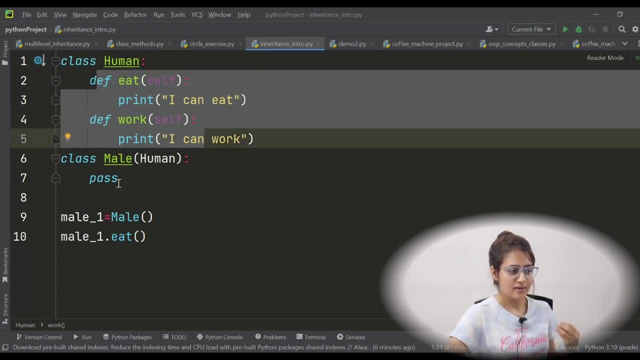 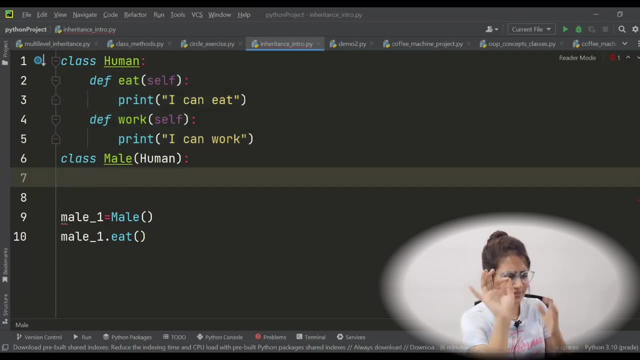 We are reusing this code again rather than writing this again, We are just reusing it Right Now. this thing, this is the simplest concept of inheritance. The second thing is this derived class can implement, can have its own attributes and its own behavior. 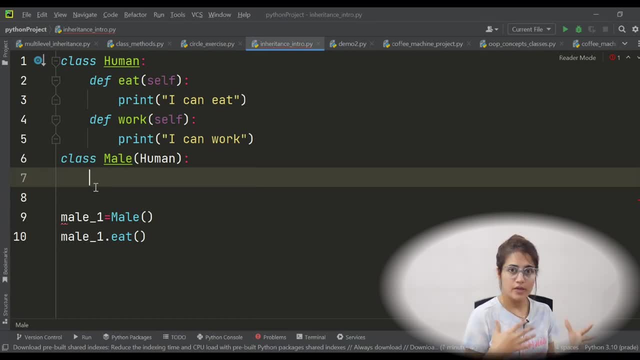 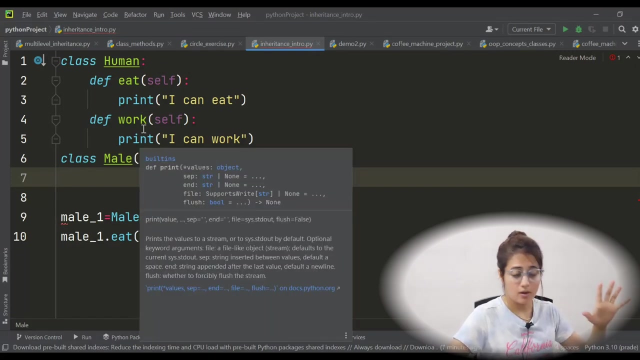 Right, Like we, We can have our own behavior. It's not like that everything, the all the properties, all the appearance properties and all the like, our behavior we inherit from our parents. No, We are having our own identity. Maybe their, their, you know, their way of doing some work is different. 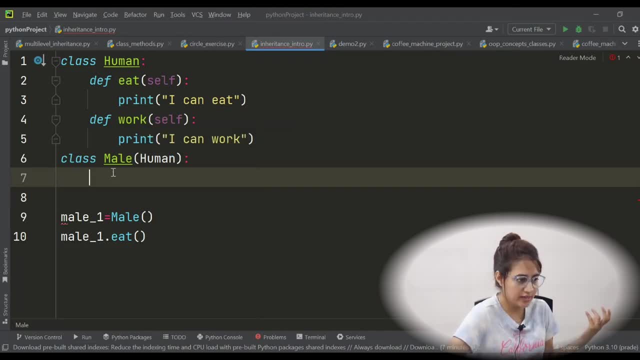 Our way of doing our work is different, So we can have different behavior. So, like this, the derived class can also have its own attribute and methods. So right now, just I'm not taking the attributes, I'm taking just methods. So I'm just defining a method. 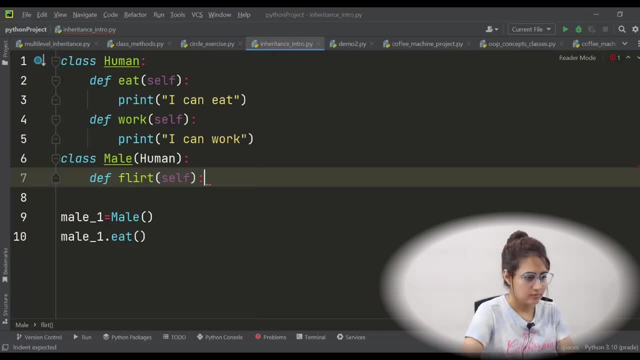 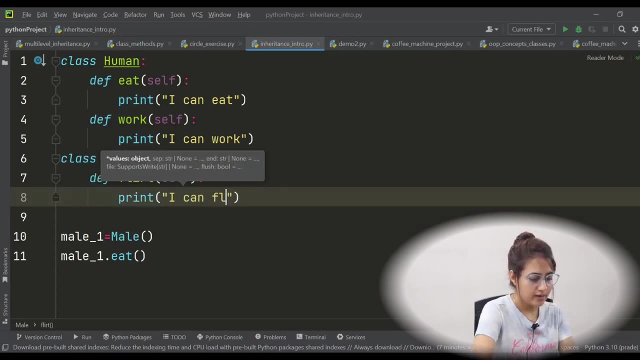 One more method like maybe flirt. No offense, It's just an example, Don't take it seriously. So I can flirt. Now see these. now see, using this male, how many thing you can access: male dot, eat and work from human class and flirt from male class. 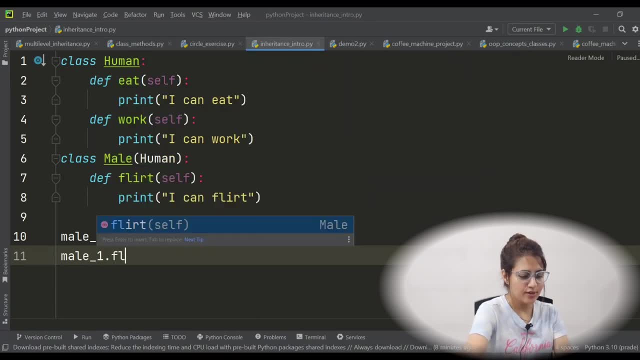 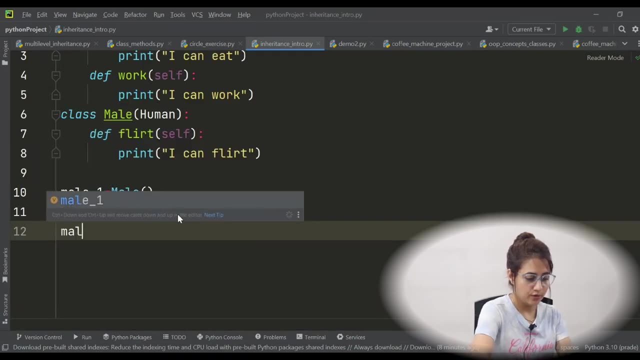 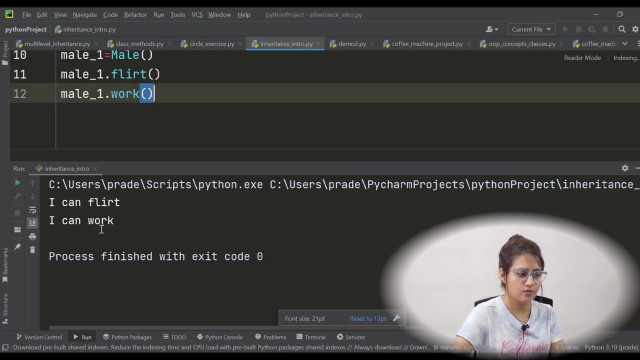 All the three methods I can access Right. So if I access this flirt So it will print: Yeah, I can flirt Right And both. if I want to access, like male, one dot and work, This is also fine. See, I can flirt. 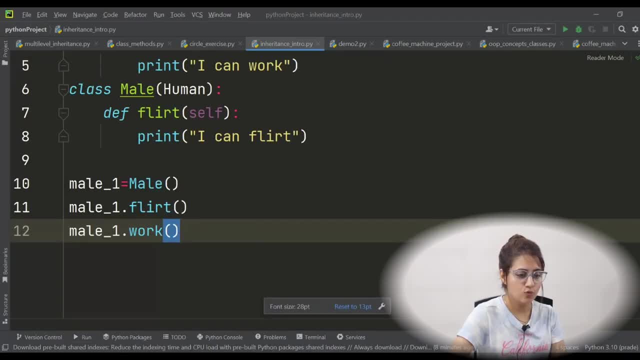 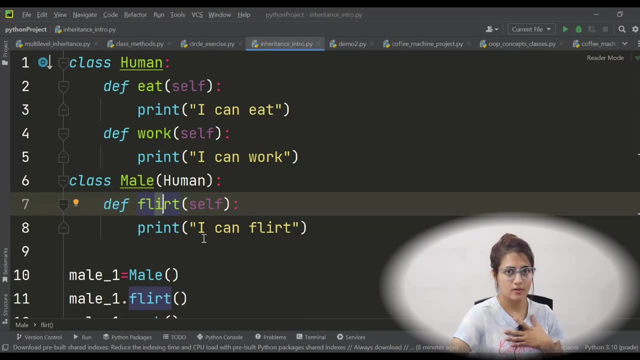 I can work Right. So this work, this may class is accessing from human and this is its own method. So our own attribute and methods we can define. This is second thing. Third point: important is This drive class can have its own implementation of the method that has that are already defined in human class. 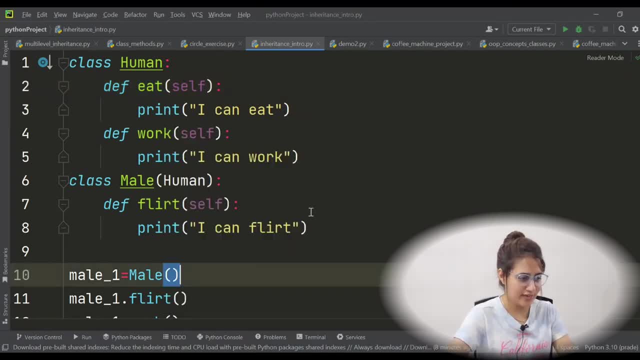 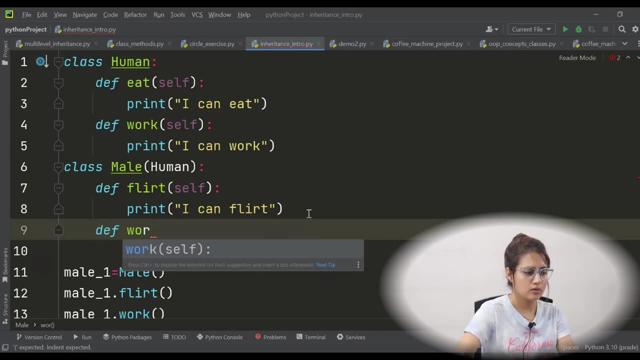 Now what does that mean? Let's see, practically cannot getting my words. See, I am taking the same method- work from human class work- But my way of work is different from human class, So I can redefine this method here. So my way of work is like: maybe I'm specific. 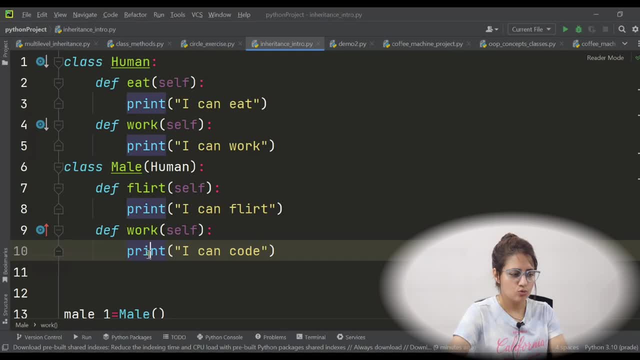 I can code, So I have. just I'm my, I'm having my own implementation of this work method And this woman class is having implementation of this work method. I can work, but I am having I can code, So this particular thing is called overridden. 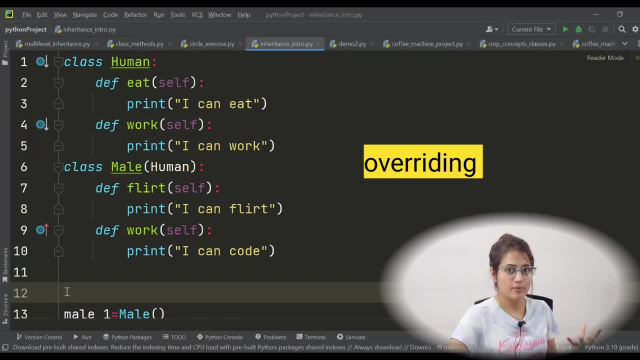 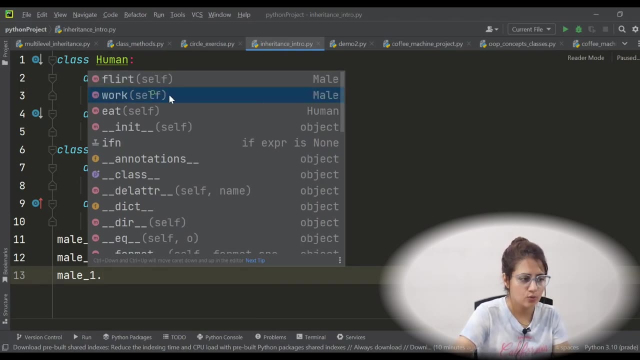 This is what Override concept method. overridden. overriding means you have overrode this method, work method previously this, but you have overrode this method right Now. if you want to access using this object, male one dot see flirt, work from male. eat from human. 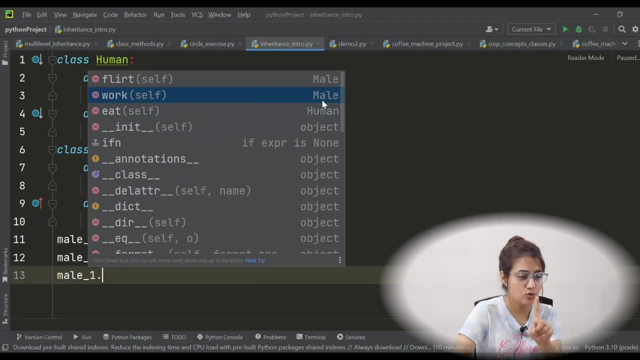 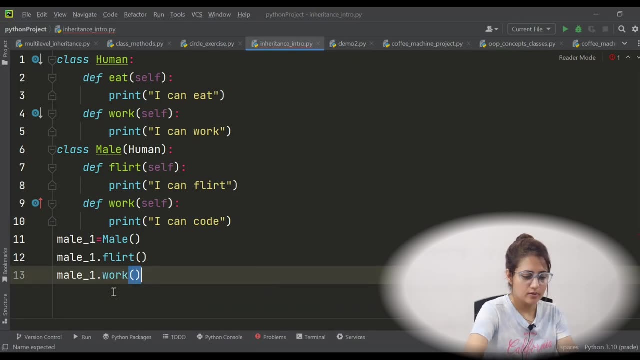 See, this work is from male You are accessing, not from human, because I am having my own implementation of this method. So if you print Work, then it will print, not I can work, It will paint, I can code, because you have overridden this method. 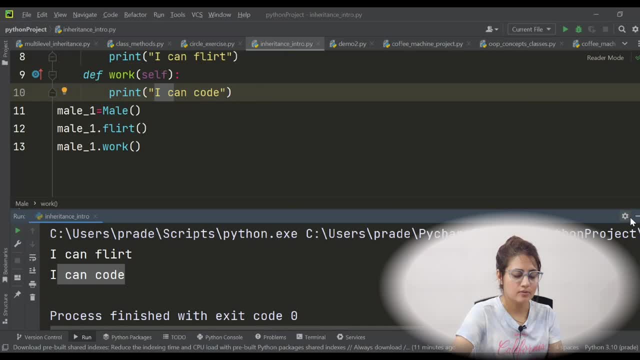 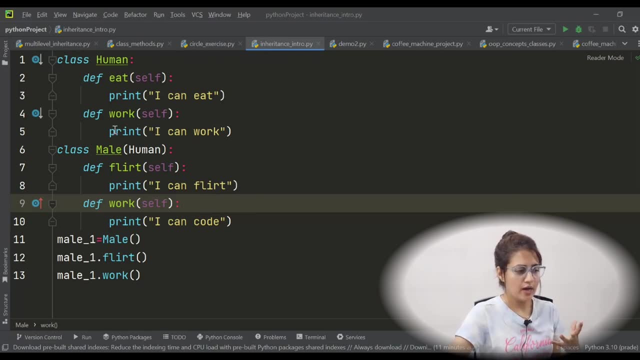 I can flirt, I can code right. This is overriding concept. Okay, fine. Now next point is: if you want, if you want to have this, this definition also, this implement implementation also, as well, as you want to add something extra In that definition of that method. 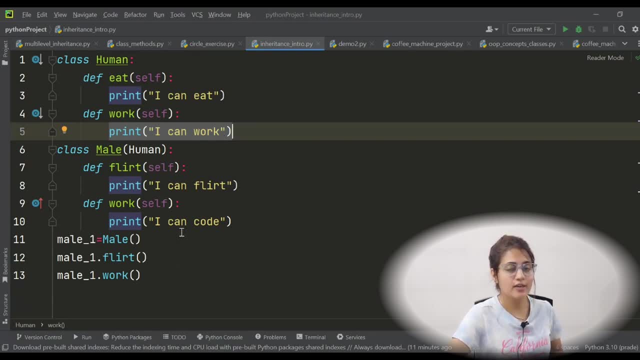 See means I want to print, I can work as well as I can code. Right, I'm not implementing, I'm not defining this method from the scratch. I want the previous definition from the base class and I want to add some extra. 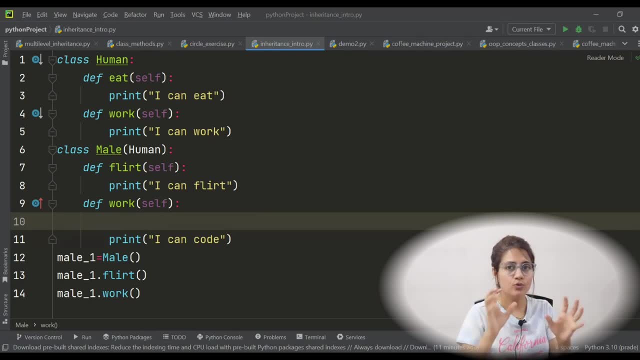 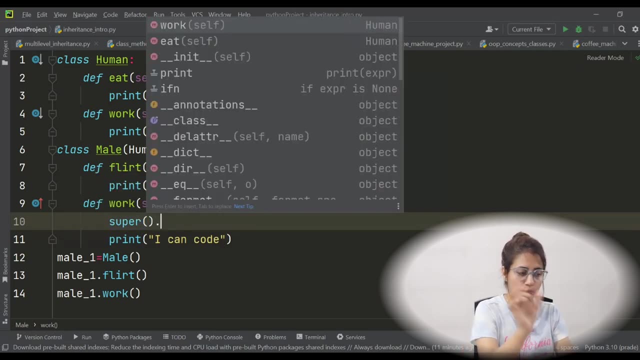 Right. So that what, how you can do that you can access with the help of. we have a function, super Super. Just call this function: dot. What method See with the help of super. it indicates that from human class, from super means super class. 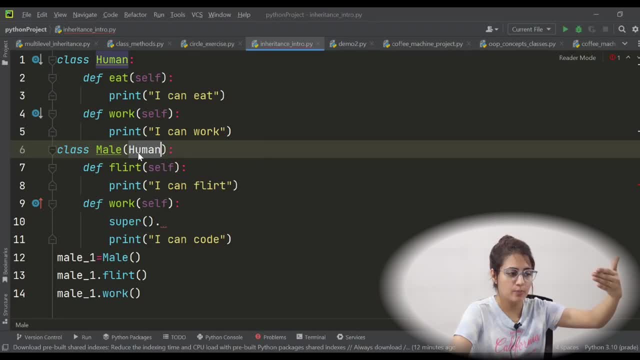 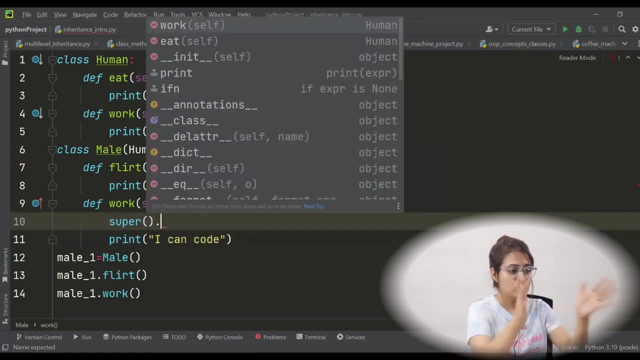 We know the base class. So base class is what class you have passed here? human. So this is human, is what the base class? So from base class you can access all the attributes and methods of that class Right With the help of the super, super dot. 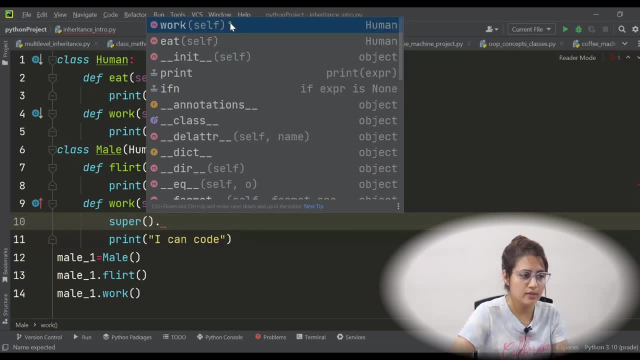 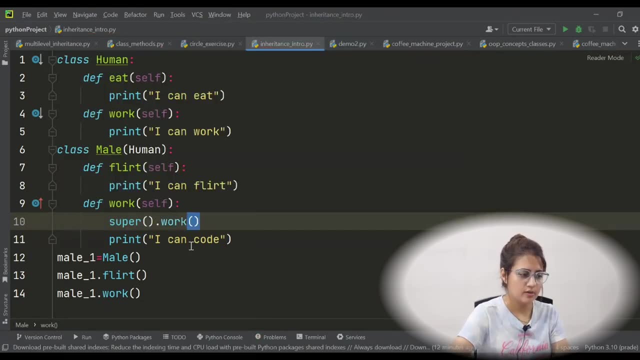 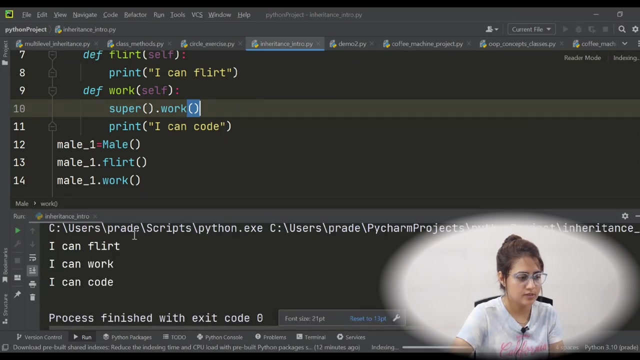 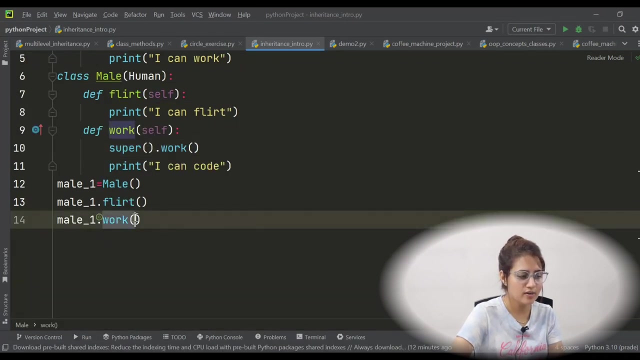 Now work, See human- and eat, So work, Sorry, And I want to access this thing: Super dot work Right Now. see, let's print male one dot work. See, I can float and I can work, I can code. Now this work definition is because we have accessed this implementation from super. 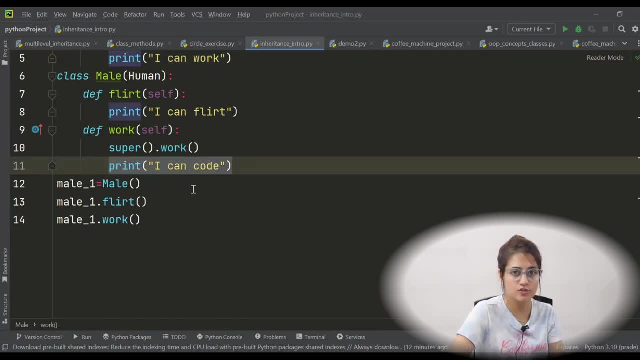 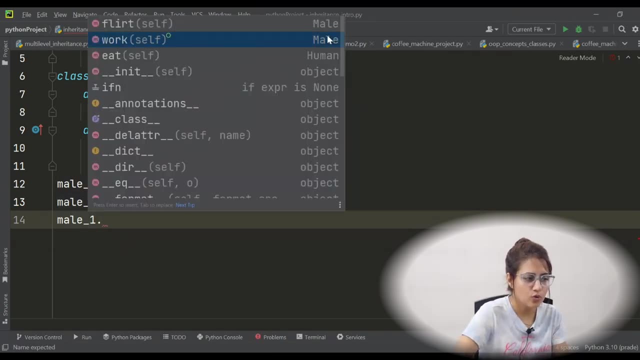 So it will print. I can work as well as now. I have added my extra feature. It's one more statement I can code, So both thing it will print. And now, if you see, here This work is from male only, Not from human. 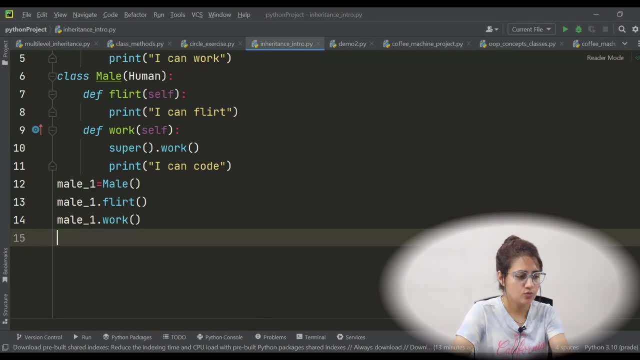 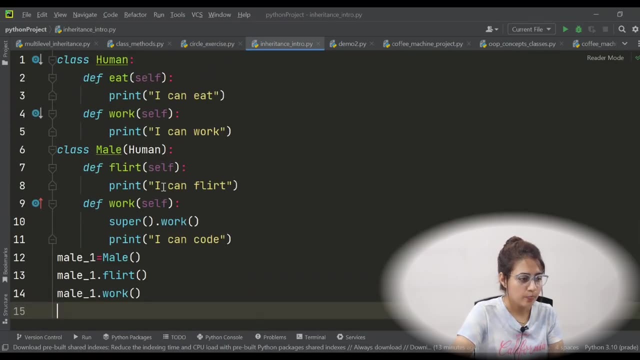 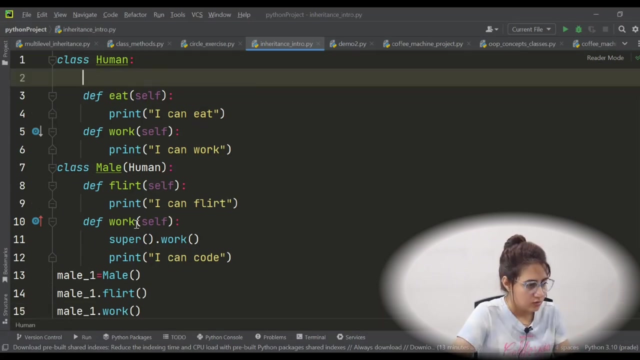 Male only Right. So I hope you got this thing Right. I can float, I can work, I can code, So these kind of thing you can do. Now this is about methods, If suppose I am having attribute two. So 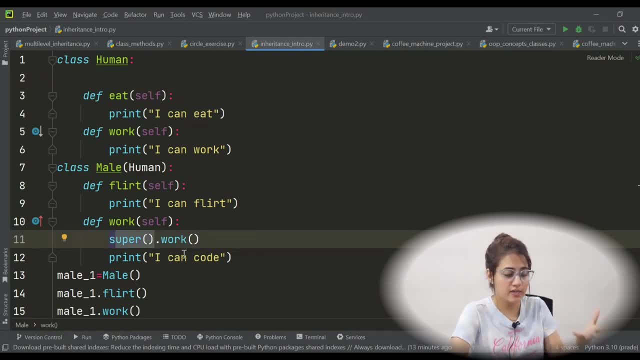 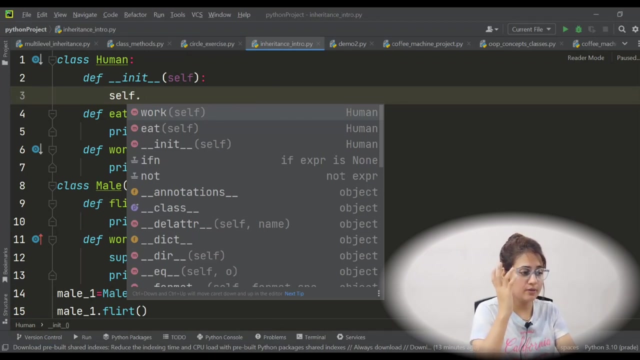 So this super class, The super function, is basically give you the access to all the methods and attributes of parent class, Right? So let's define some attribute also. I am having a init function And there I am having like two attributes. All the human are having like maybe two eyes. 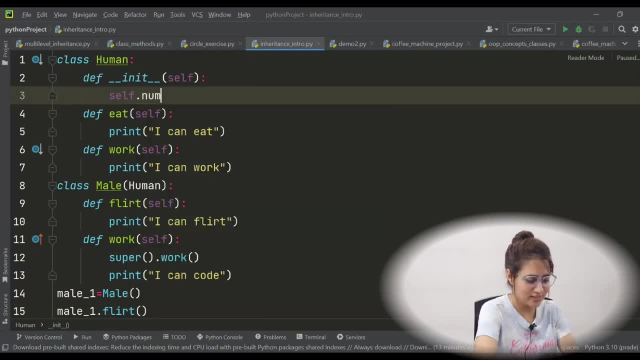 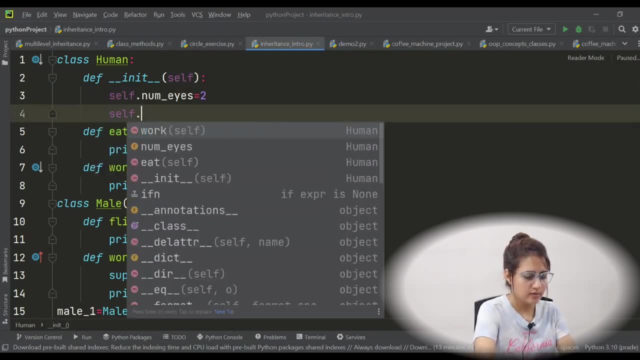 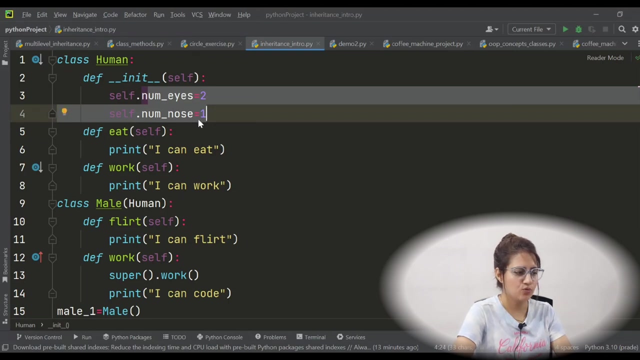 Maybe not, Not maybe, Yeah, definitely. they are having two eyes. So num underscore eyes equal to. I am setting two, Right And Nose. Number of nose equal to one. Only two attribute: I am taking Number of eyes and number of nose. 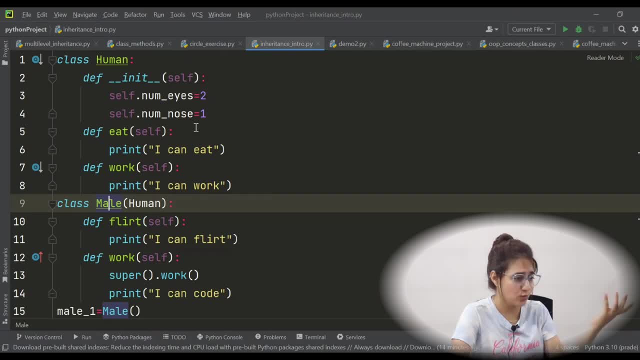 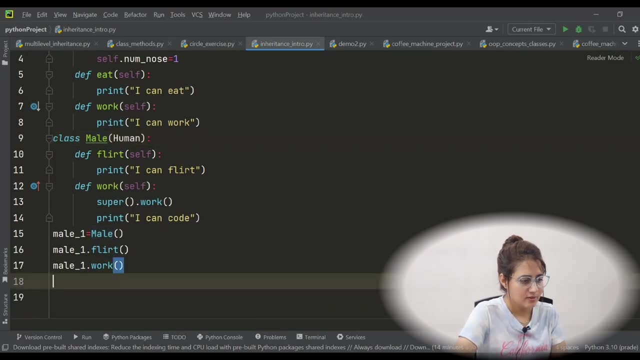 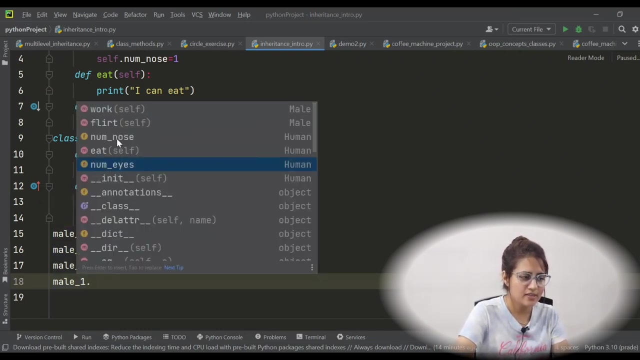 So obviously male is also having the same thing: Number of eyes and nose, Two eyes and one nose. Right Now. see, With the help of this male object, Now you can access num. eyes and number of nose From human class and number of eyes from human class. 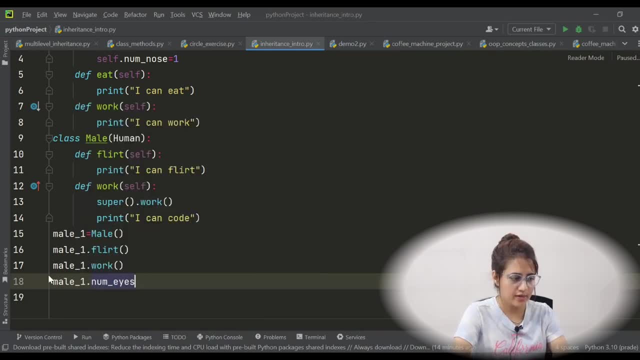 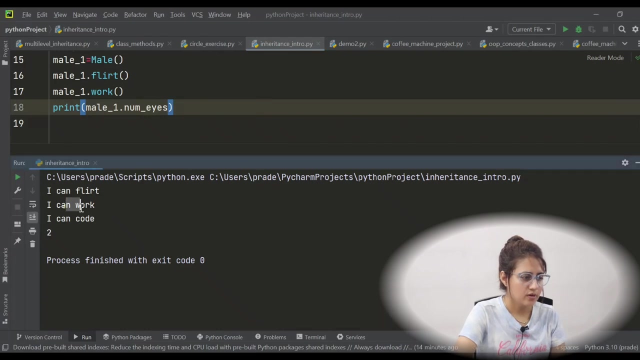 Right. So if you want to print num underscore eyes, I want to print this thing. So let's print How many number of eyes this male object are having. So let's run this and it will show you. See, I can flirt. 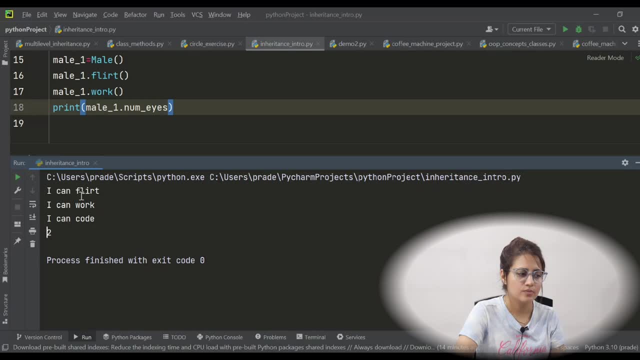 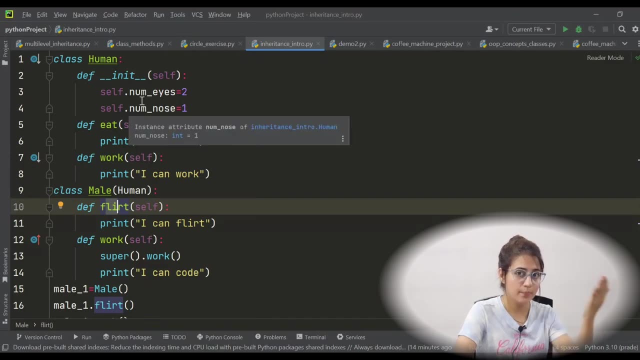 I can work, I can code. and number of eyes are two, Number of eyes two. We haven't defined any attribute in male, But it is accessing from parent class Right, Like this: And if Now, rather than eyes and nose, 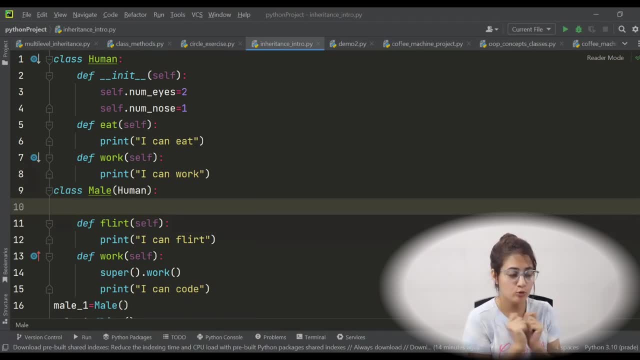 I want to specify one more attribute specifically for male, So that also you can do With the help of def. I want to Initialize and, like I want to pass one parameter Name, Name of the male With this class Right. 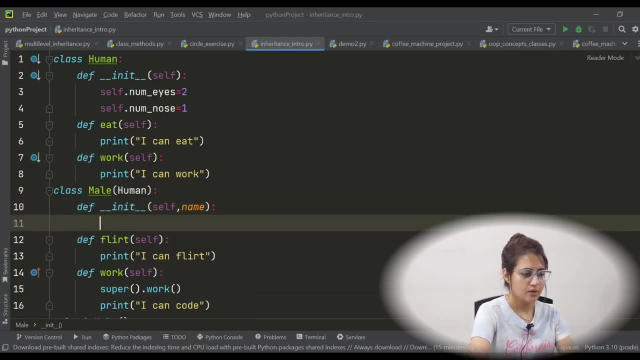 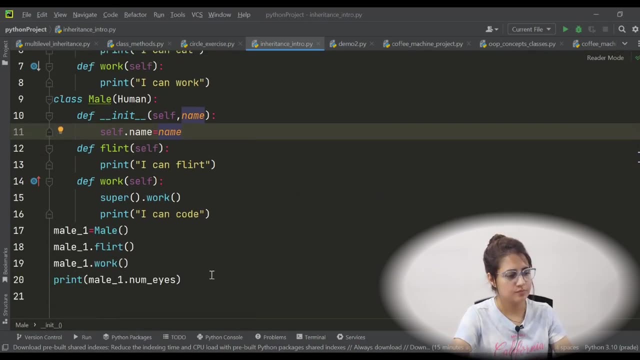 So while calling this now creating object, you have to pass Name. So I am writing Like self dot. Name is equal to Name. Right Now it will give error While calling this object Because See In line number seventeen. 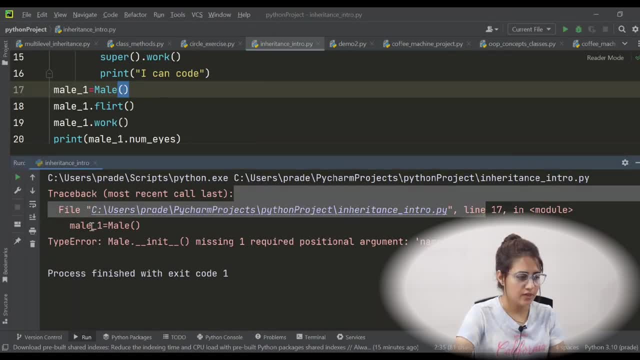 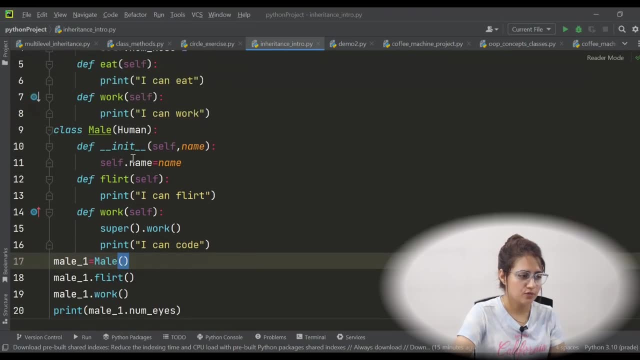 While you are creating this object: Male type error: Male init missing one required positional argument Name, Because in defining In this Constructor You have to pass This parameter name. So let's pass This name, Maybe, Akash. 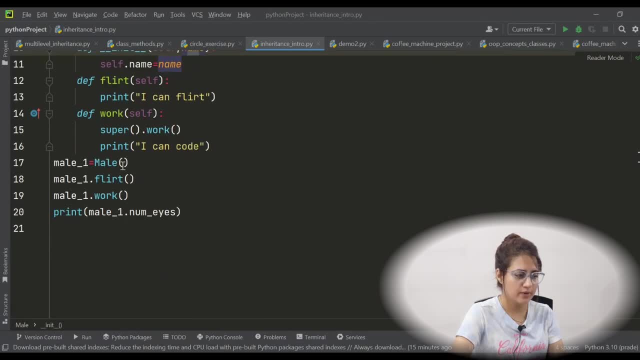 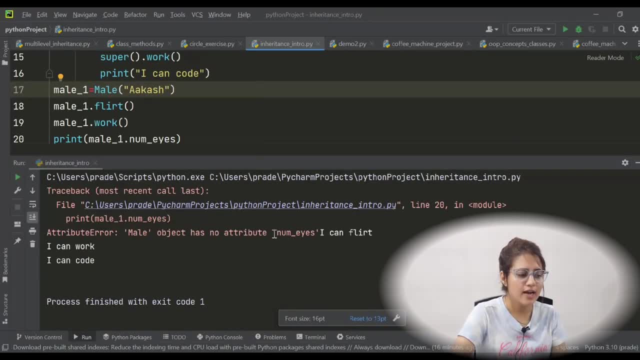 Maybe Akash, Maybe Akash. Let's run this Now. Male object has no attribute num eyes. See No attribute Num Eyes. Why so? Because See Last time, In line number twenty. Because you are printing num eyes. 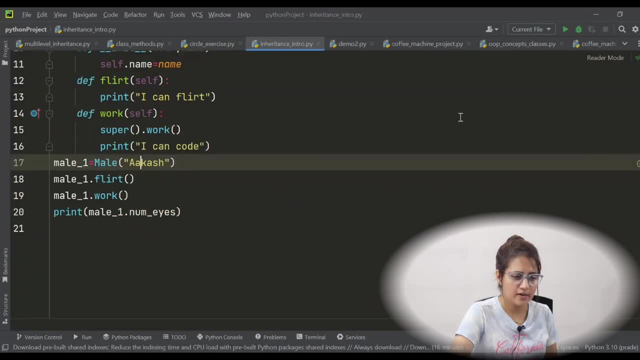 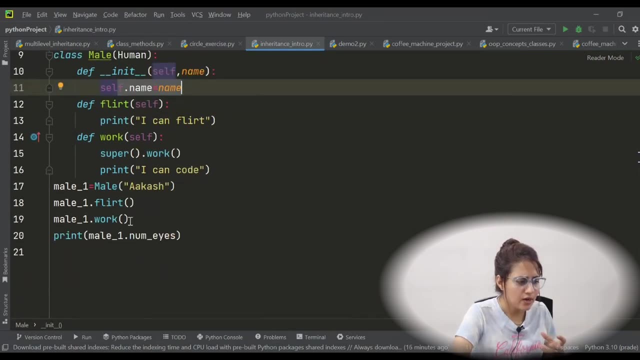 And male object is not having attribute num. eyes In male object. Now I am having only Name attribute, Name Attribute, Name Attribute Name. But see, Now, at this point of time, Let's see, Let me just show you this thing. 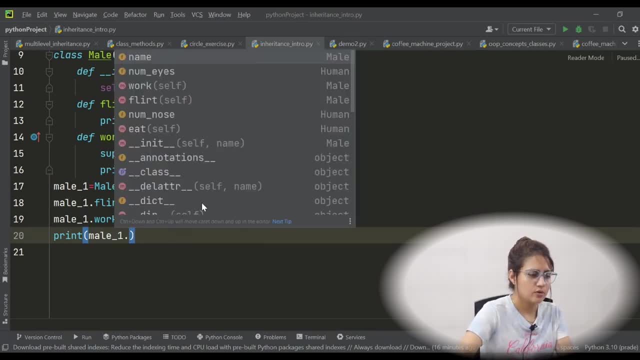 If you want to print Male one dot, Then name Num eyes. Num eyes are from Human, Number of no's from Human. Maybe you think you can access. Let's access number of no's, So Maybe you think it should print. 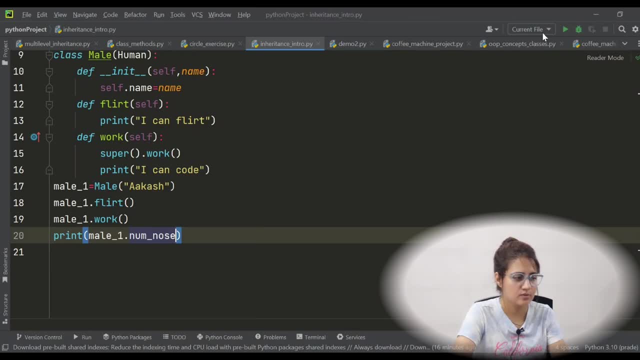 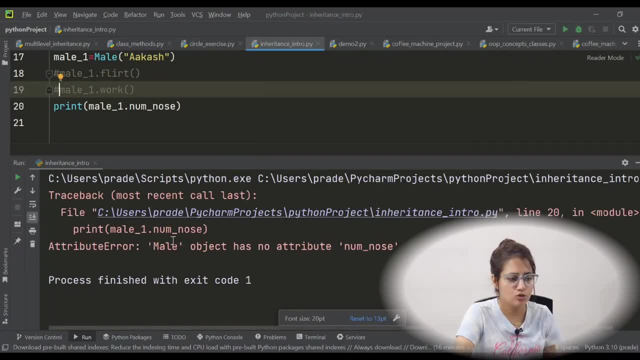 Number of no's. Number of no's. See, It is not printing anything. Male object has no attribute. Num no's. Why you are getting this attribute? Because this is derived class. We can access all the attributes from here. Because now? 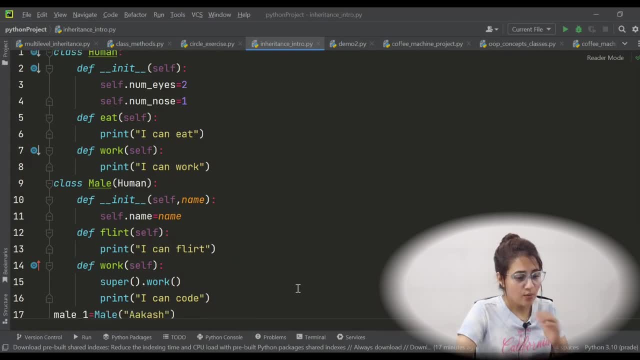 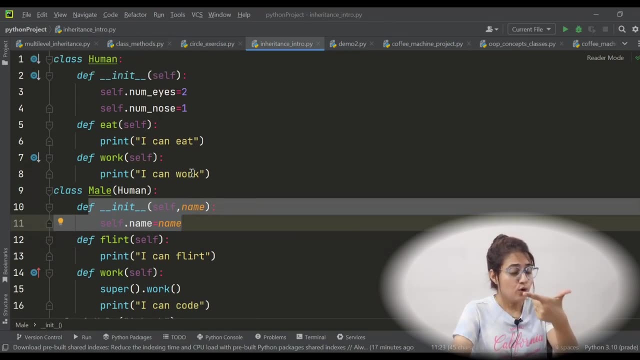 You have defined Your own init function here Right Now, If you want to access These attributes. If you want to access these attributes, Then you have to use Super function. So Yeah, We can use These Attributes. 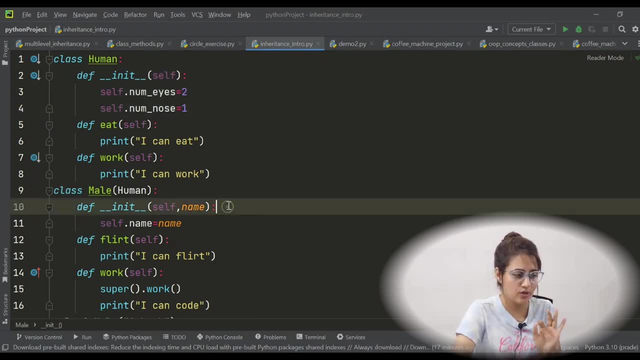 If you want to access these attributes, Then you have to use Super function. So Yeah, We can use These Attributes As well, But for that In this Init function, In this Drived class Init function. 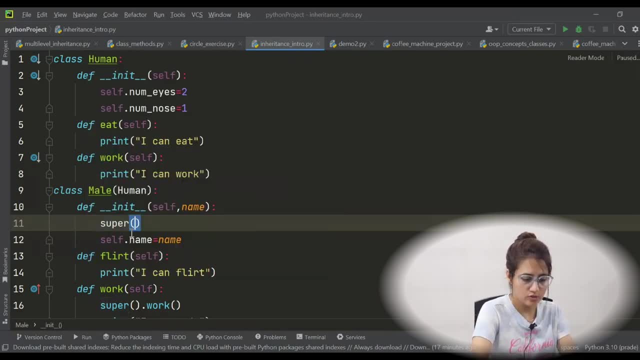 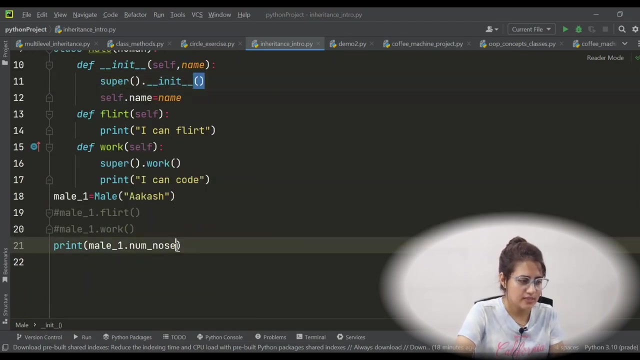 You have to call This Super function, Dot Init, Init function of Super Right. And Now, That's fine. Now Let me just Run this: See If, Again, Male One Dot. 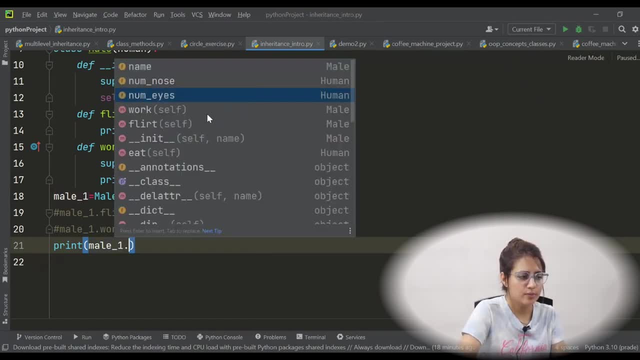 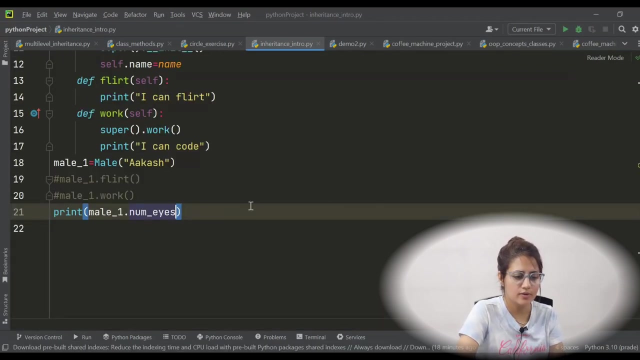 Name, Number of No's, Number of Eyes From Human And Work Float And These Are The Methods Eat As Well As From Human Right. So Number of. 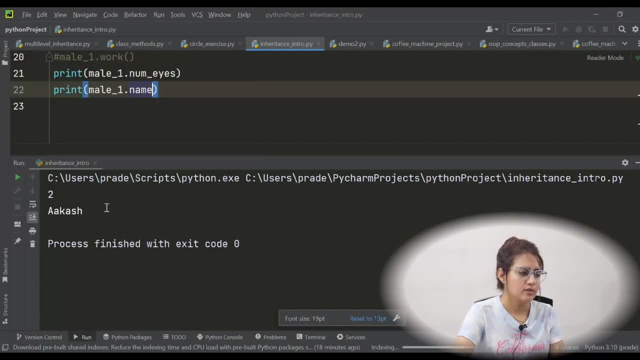 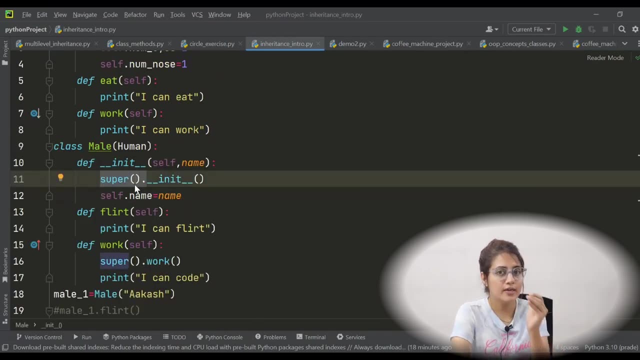 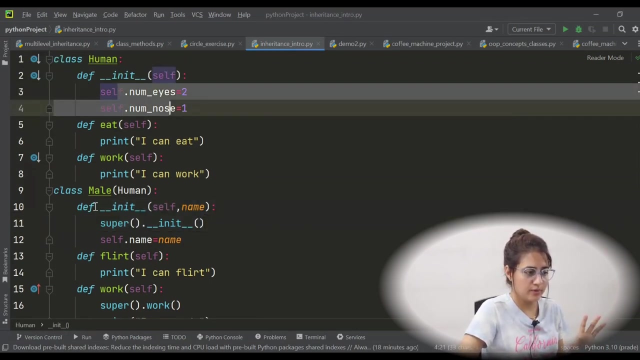 No's Or Number of Eyes. I Want To Print This Super Function. It Will Give You The Access Of All The Attributes And Methods Of Super. 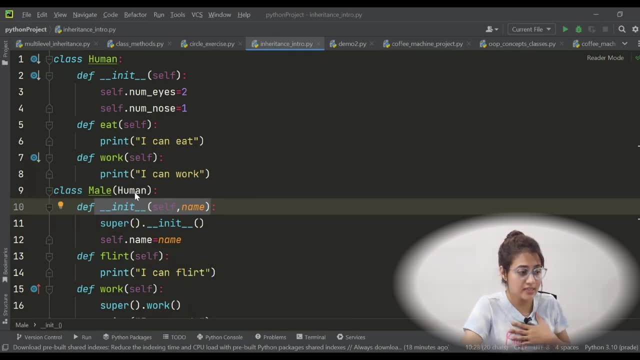 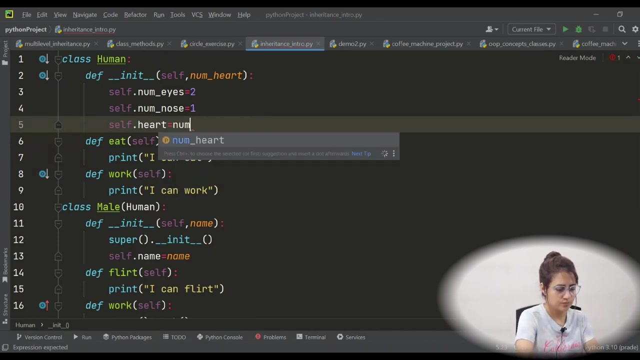 Class Right, Because Here You Have, If You Don't Define Your Own In Case, Here Also I Want To Pass One Argument Like Maybe Self. 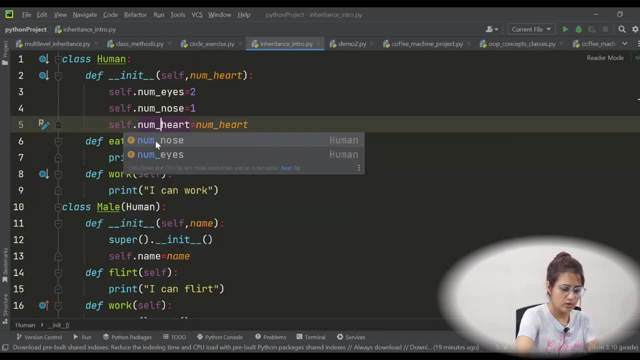 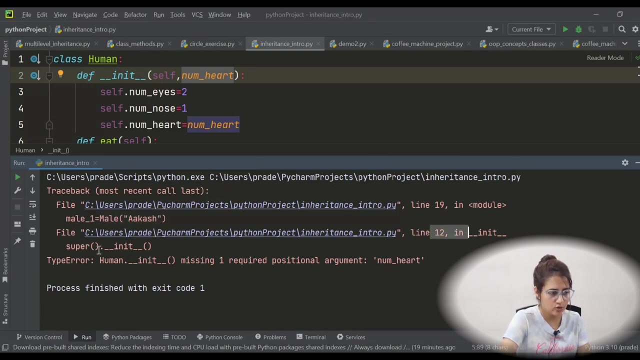 Heart Equal To Num Heart, Or Maybe Self Heart Or Num Underscore Heart, Num Heart. Right, You Have One Parameter If You Run This Like: 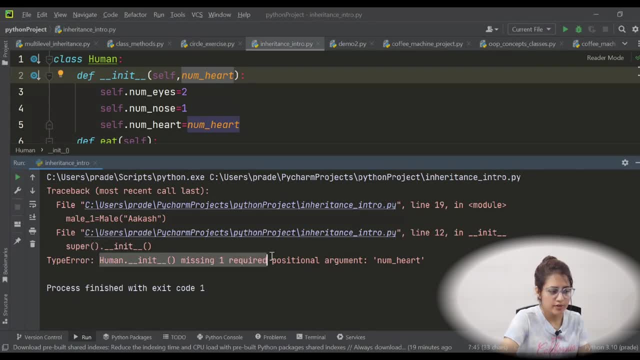 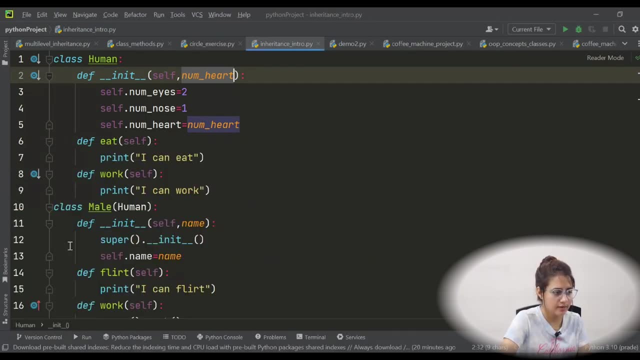 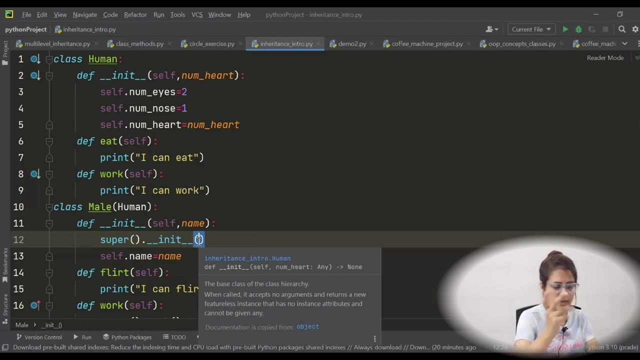 This See In Line Number Nineteen, Because You Are Calling This Akash, And In Line Number Twelve, Super Init. This You Have To Use. 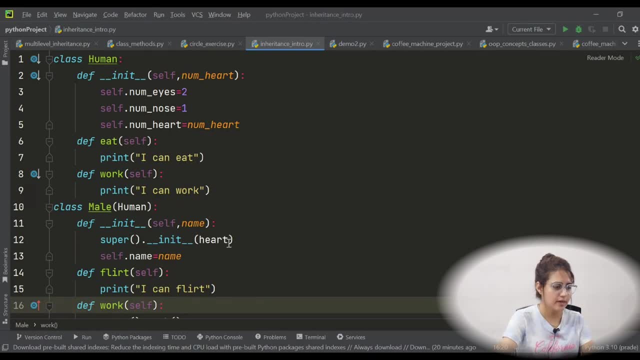 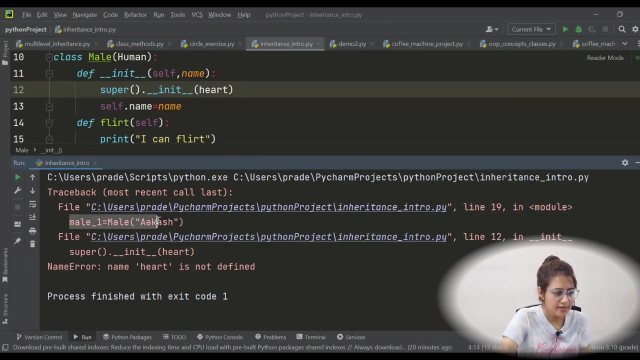 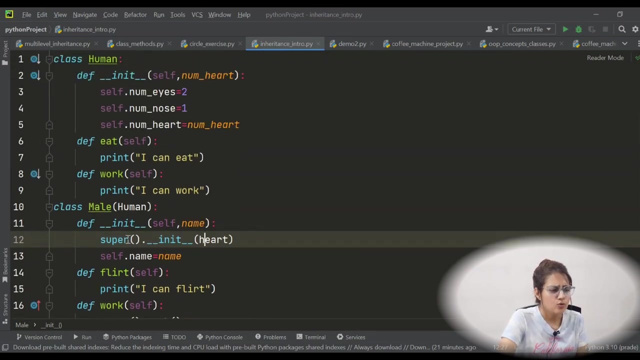 This Num Heart, Same Name, So I'm Calling Suppose Heart, Only Heart, Right, Okay, Still It Will Give An Error. See Now, Maybe You Think. 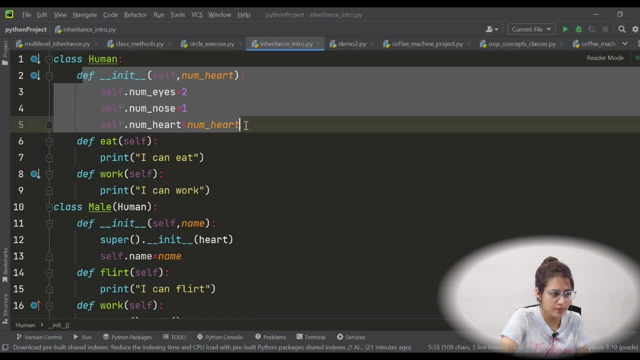 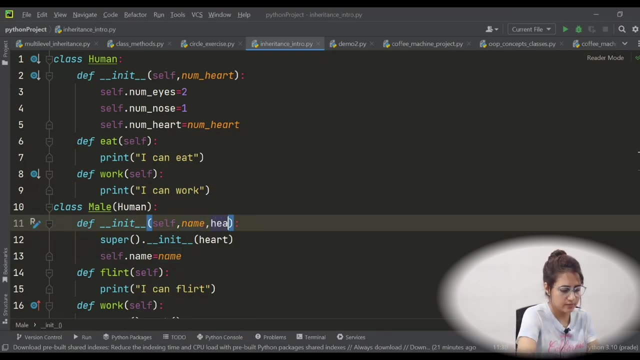 That You Are Accessing All The Attributes From This Human Class. Right Means One Parameter Is Number, So Rather Than Name, One More You Have. 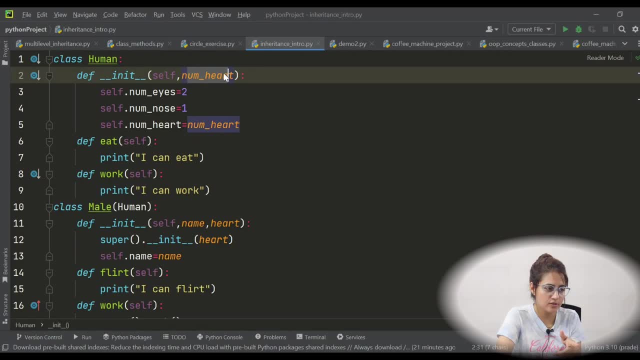 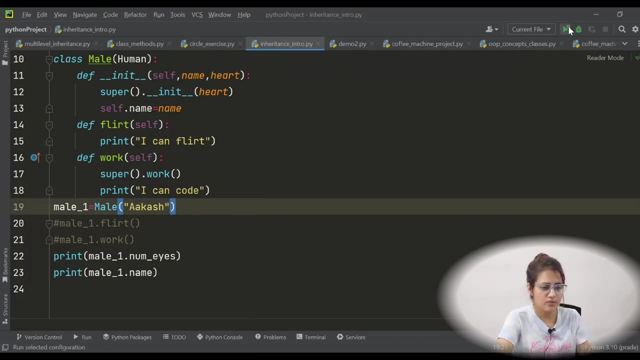 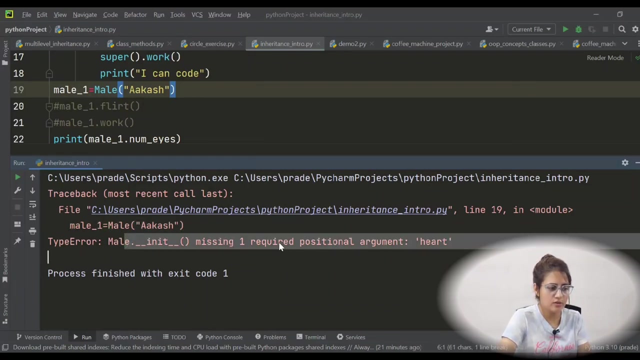 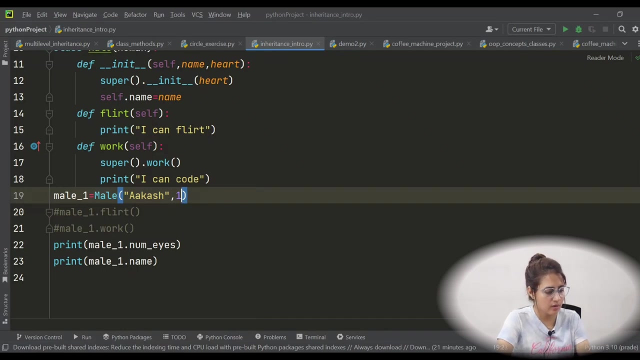 To Pass Here One Parameter. This Can Be Different Right Now. It Will Work Fine. No, It Will Give Error, Because Akash As Well As 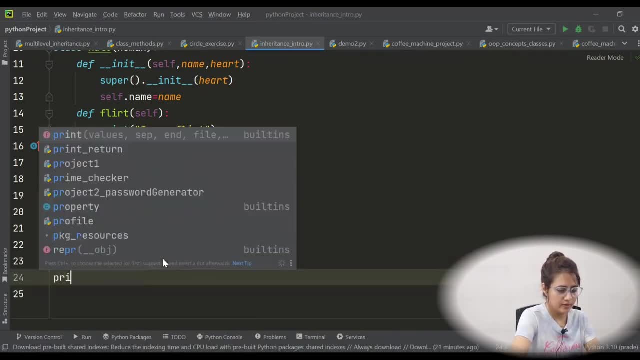 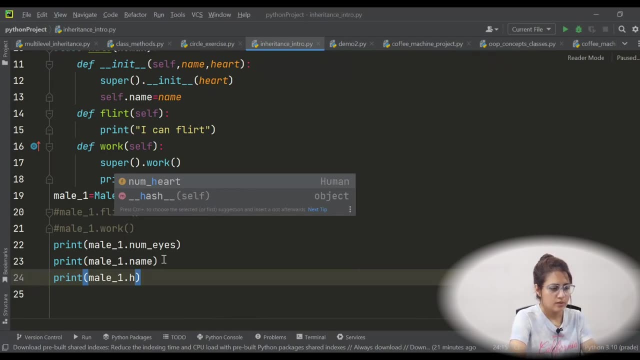 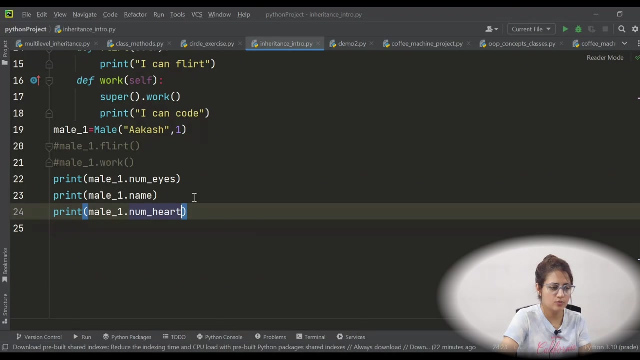 Okay, Let's Run This. Whatever You Will Get Dot See, You Can Access Now Num Heart This Attribute Of Human Class. So Num Heart See. 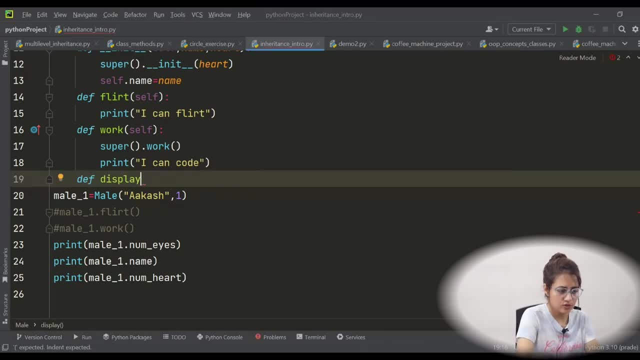 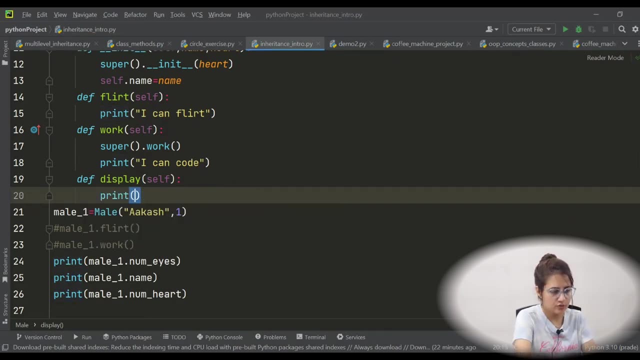 Num Heart Is One Name Is Akash. And Number Of Heart. Using F String Like Hi, I Am Name Of This Object On Which You 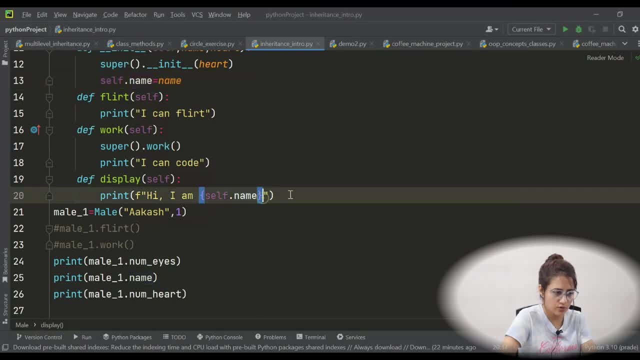 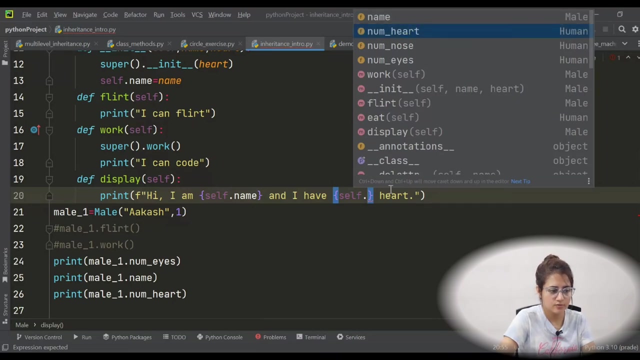 Are Calling, So I Am The Name. Obviously We Can Fetch With The Help From Where You Can Fetch The Value Of This Heart? From Self.